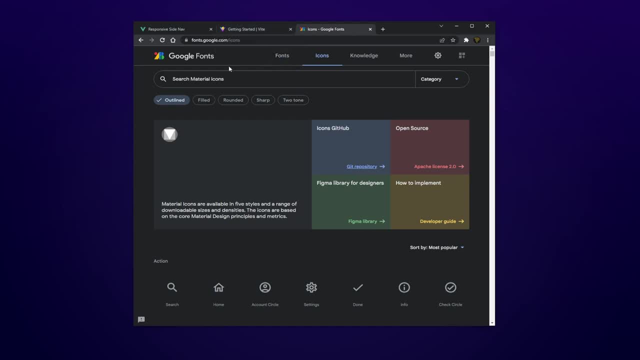 It's super simple. It makes few development ten times faster, and we're gonna be using Google icons as well. So the material icons, and I'll show you how to get set up of that as well. So, without further ado, let's get into the code. 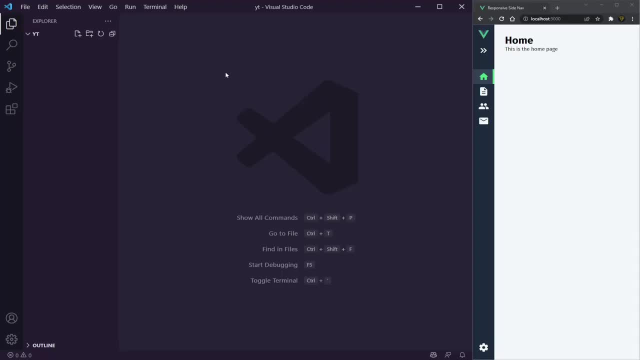 Okay, guys. So I have opened up a new folder inside official studio code and we it's just an empty folder, Nothing special about it. you know that, that's it. That's all I want to show you for that. So we're gonna open up the integrated terminal. You can see it's a toggle terminal. 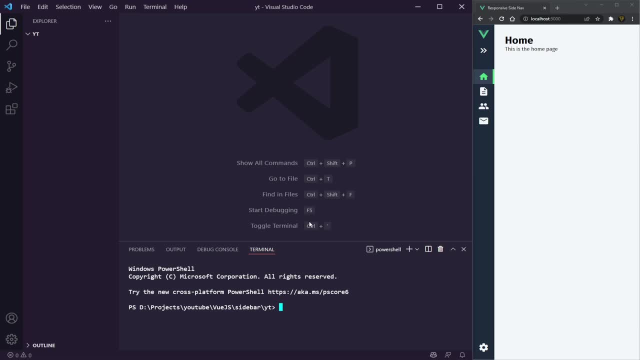 It's control and apostrophe, but this probably be different on a Mac. I think it's control Options, or, yeah, control options. T on the back by default, but yes, so now we're in our folder here. now we're gonna get side with a. 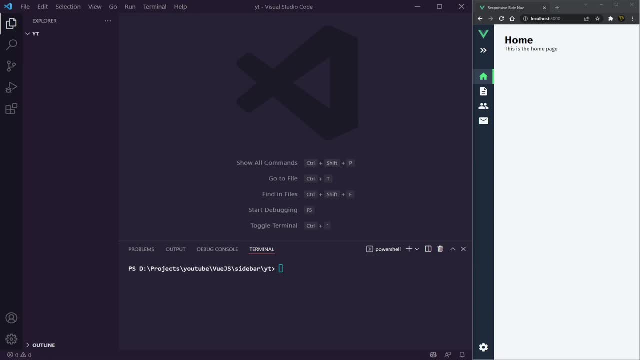 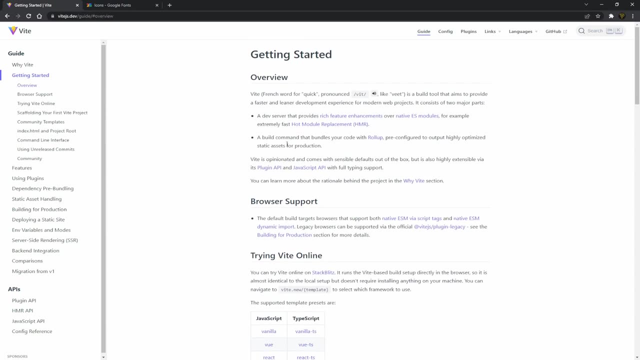 Fight tool. so I'm gonna show you how to set fight. now, If we go to the browser, you come to this page- fight Js Def forward slash guide- and you can give you an overview about how you get set up with fight. I'm gonna be you to this. you can see your MPM create. 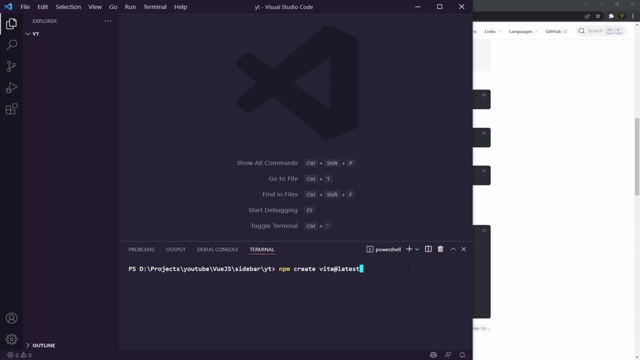 Fight at latest. so if I copy this, So inside here, if we just run MPM, create fight at latest, and then we can give it a project directory, So we can say dot, which means the current directory win. You can also give this a name, set, say sidebar, and this would create a folder inside the directory. 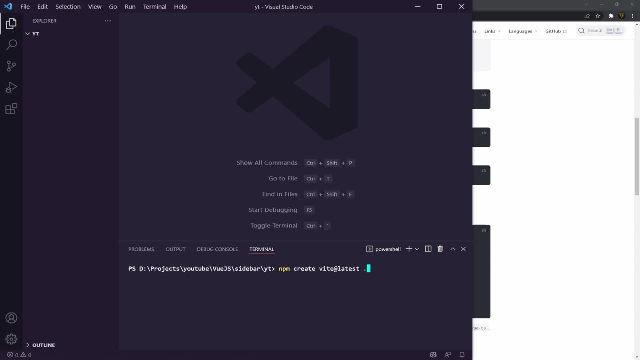 You're in called sidebar and pull it all in there. Well, I'm just gonna say dot, and then we could also give it a template. Let's say few like this, and that would get us up with you. However, you don't have to type that. it's a lot longer with it. 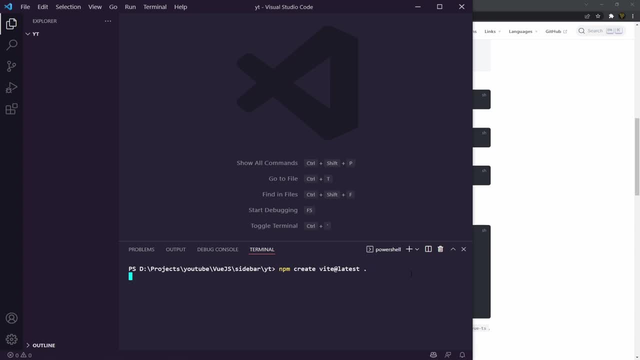 and it's gonna Ask you anyway when you hit enter. so let's try it this way. So if you enter, it's gonna be like, hey, what's the package name? now, This is just your package dot JSON file. I'm gonna call it package dot JSON. I mean, it makes sense, That's what I want to use. 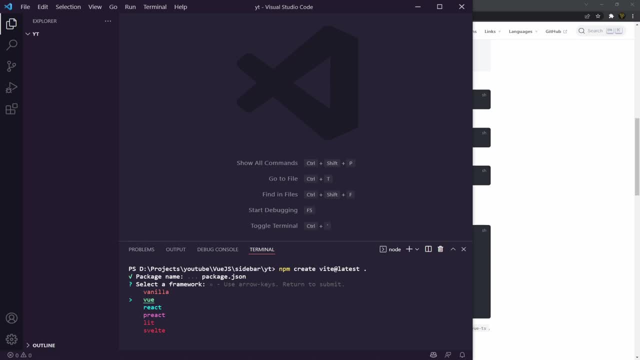 You can see a select, a framework. So obviously fight isn't just used for few Js, But in this tour we're gonna be using few. you can even use it for vanilla java script Few Js, react, pre-act, lit and it's felt, and I'm pretty sure you can get a typescript version of all of these as well. 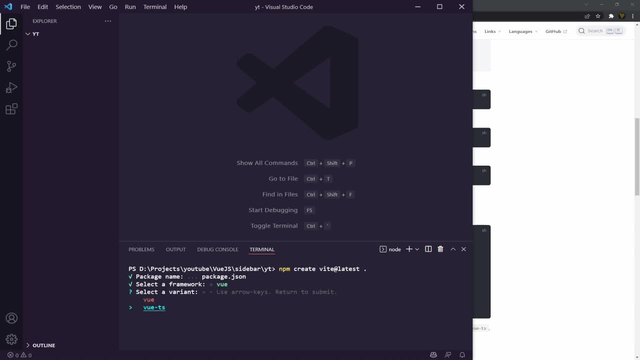 So if I hit few, you can see it says Select a variant. you could have few typescript or just few. I'm gonna hit few and there you go. That's it. See how fast. that was Absolutely lightning quick and is already set. now, if this is your first time running a fight, 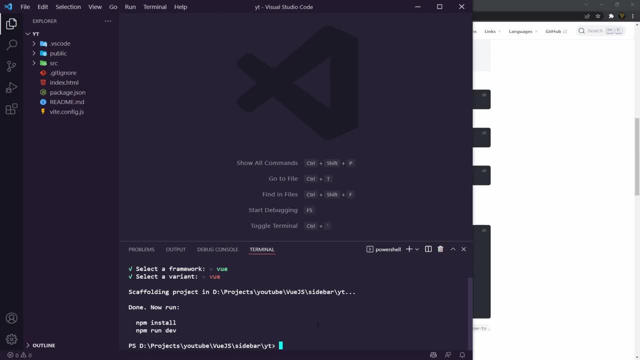 It may ask you to install a package. if it does just hit yes, it's installing some fight to make this quicker And there you go. So let's just clear this. and now we need to install our package dot JSON folder here. So to do that we're gonna say MPM I or install, it's up to you. 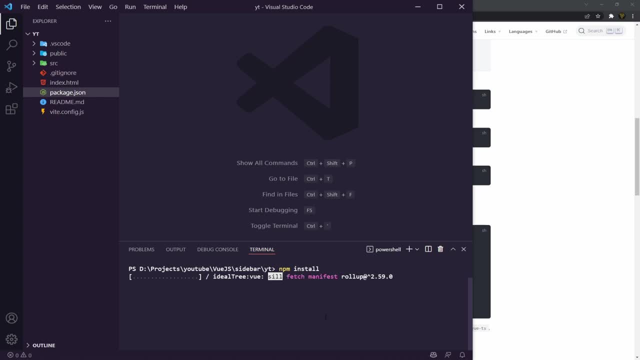 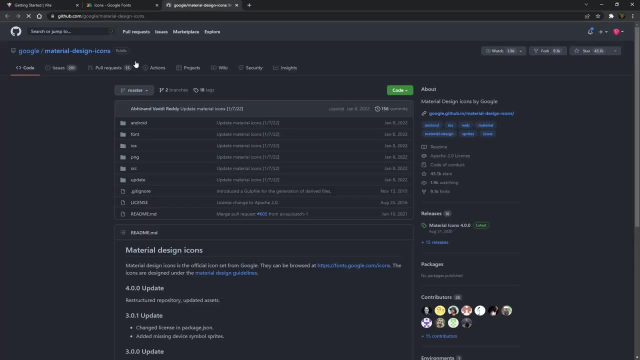 Which one you type out here: enter and that's it. It's gonna install the dependencies we need. now, while that is installing, I want to show you the Google materials to how to get that set. So we're going to click git repository here and I'm gonna scroll down to this font: stock Google the API's. 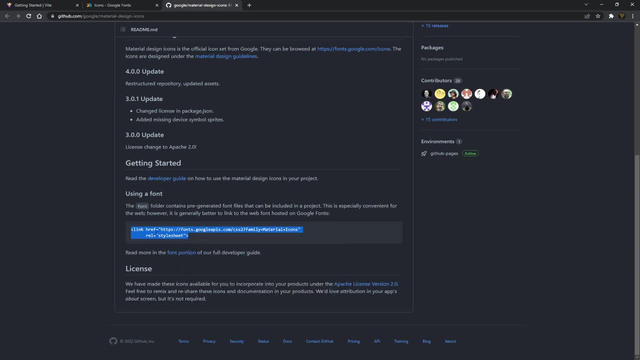 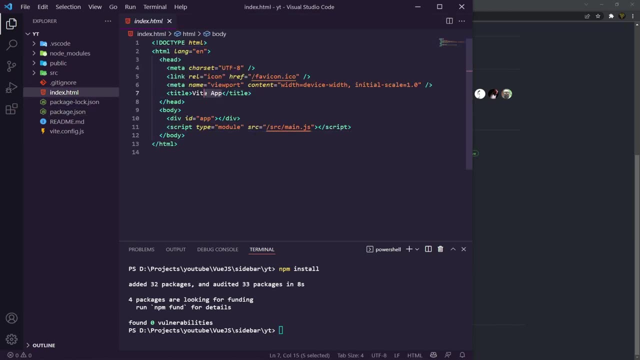 I'm gonna hit copy, copy, Just copy, copy this whole thing. I want all of it and we're gonna go back to our code and we're going to go to into our index or HTML. Then this is the root file. This is basically where our Our source app is going to connect to our app and if you can see here, title: 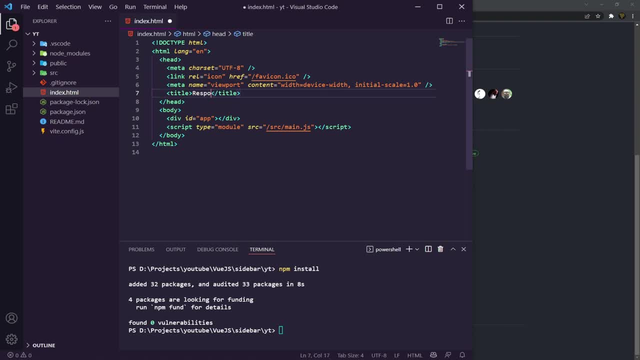 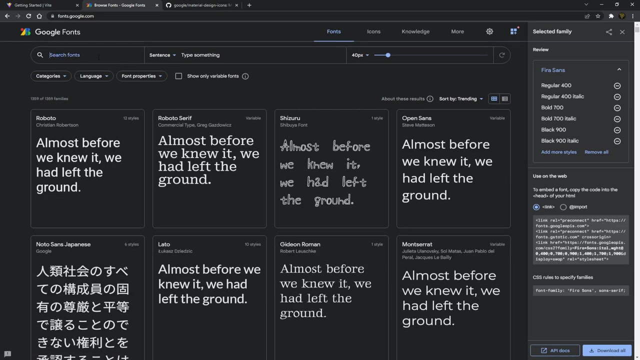 We could name this, let's say, respond responsive view sidebar, and then we want to connect our Google up right here, just like that. and Let's say we want to also get some Google fonts as well. Let's just go here and let's just search for fire of sands. 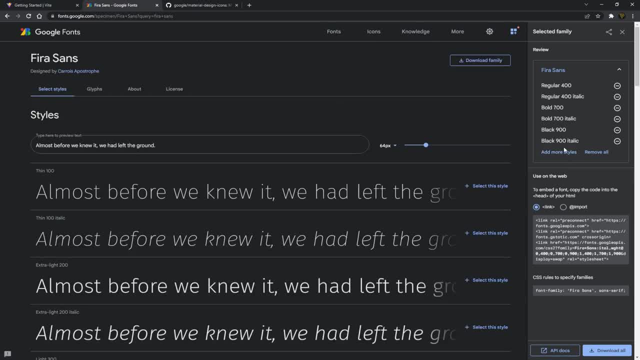 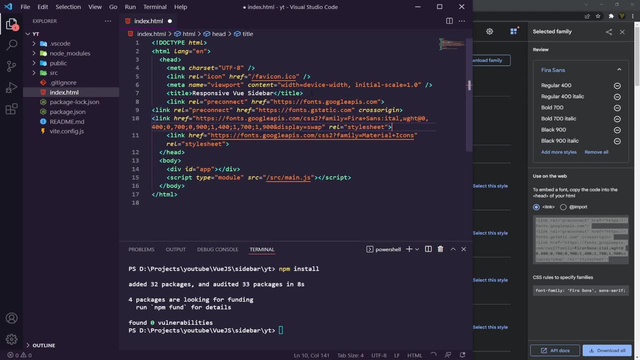 The one I always use, and on the side you can see there's some stuff set up. We could just copy this whole link in here. copy that, move back into our code And I buff the. I'm gonna do a buff the icons. We're going to use some pre connects to connect to Google and cheese static and then we're gonna get the font as well. 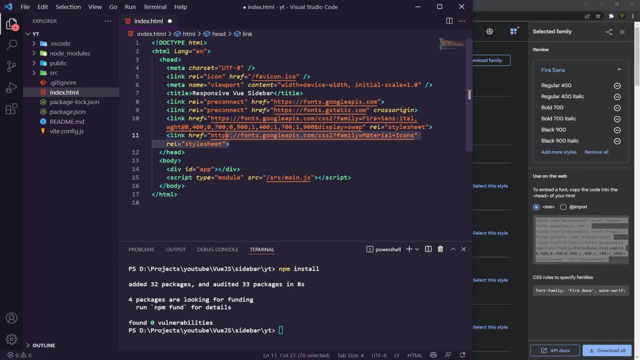 If you don't want to install a font, you can use any font you want. You don't even have to use the Google Material icons, although it does help. I'm just gonna save that, and now, once that's all done in here, We can close this as well. You can also see our packages have been installed, which is awesome. 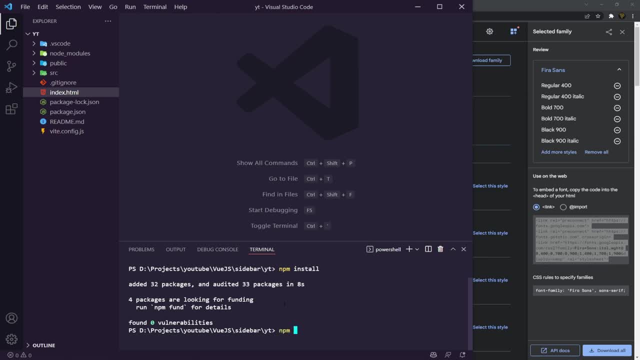 But I want to use SAS for this project. now, guys, If you want to use CSS or anything else, you can. I just want to show you how you can install SAS, because it'll be a lot easier For the styling which we'll be doing. so it's gonna be quite a bit of styling to get our math bar working and SAS just. 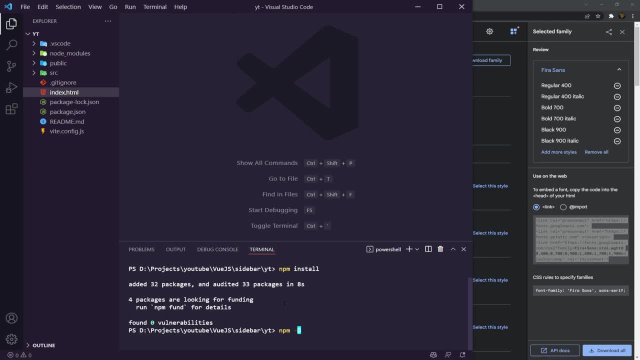 Make it easier. So we're gonna say MPM, point for D, for Add Hyphen D, and then we're gonna say SAS, now, normally you'd install it. if you do ads in fight, it adds it to something I think I don't know. That's just what the documentation told me to do. So I'm just telling you what it told me to do. 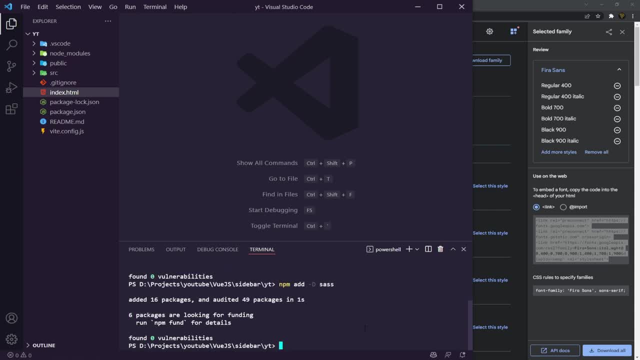 So I'm gonna hit enter And now it's gonna install SAS for us, and that's all we need to do to get SAS working. now You don't have to use this. you can use anything you want. I just want to show you that working and the next thing we want to install it's gonna be few. 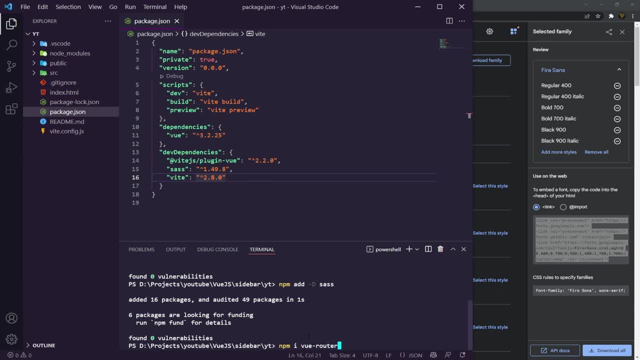 Hyphen router. now, obviously, few router allows us to have pages and stuff like that. It's not installed by default. It doesn't give you the option when you install fire fight, Compared to the few CLI. but it's super simple to set and I'm gonna show you how to do that. 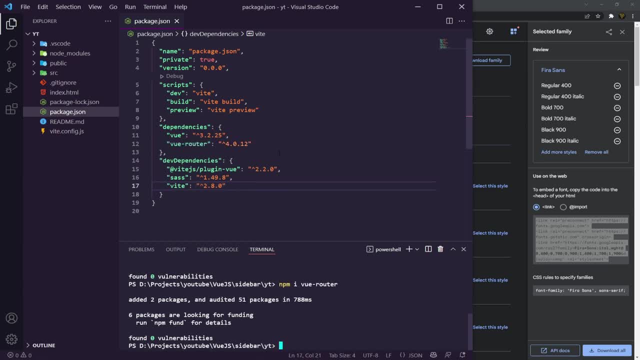 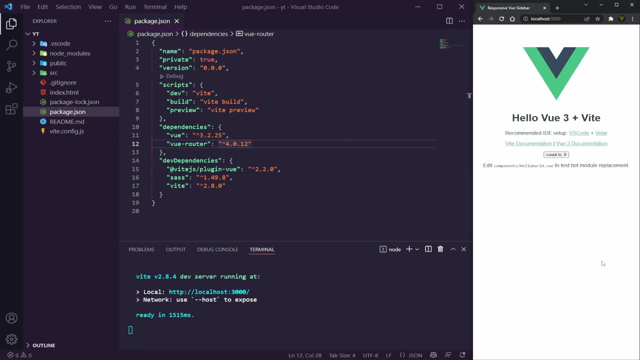 So let's just hit enter and MPM few router, You can see, is now in our package file there. Perfect. The next thing we can do is we clear MPM run death and there you go. This is the default. few free. add another surfer running on three thousands. 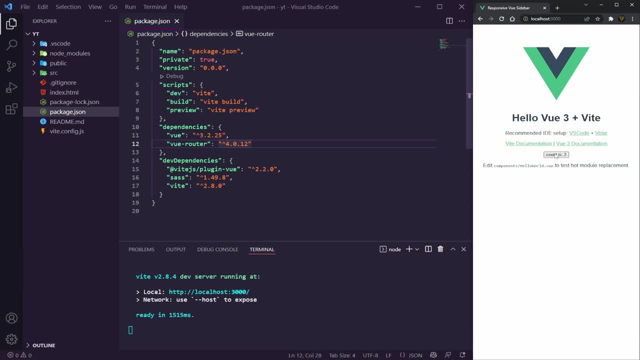 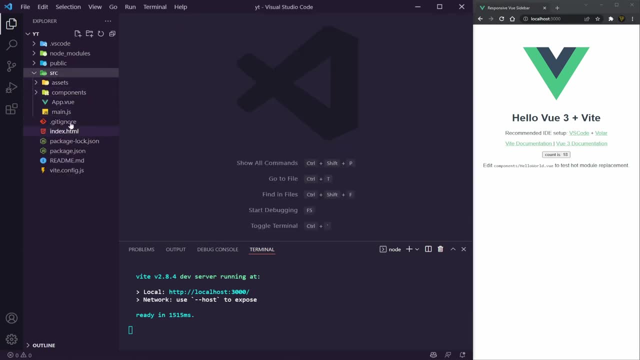 I'd to turn it off to get this to work. and there you go. So this is where I see you. we can count up, So let's go in and just get some resets done. So I'm gonna go into our source. This is where we're gonna be doing all the work for our app inside here. 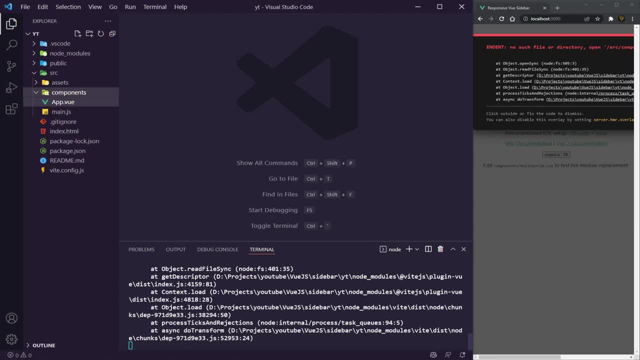 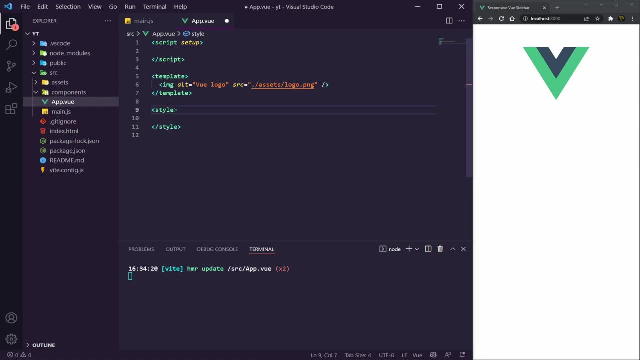 We're gonna remove the hello world component. It's not needed. Yeah, we're gonna get an error, but that's fine, we go into our our appvue. we could delete this here. it's really awesome. we're going to delete this and we're going. 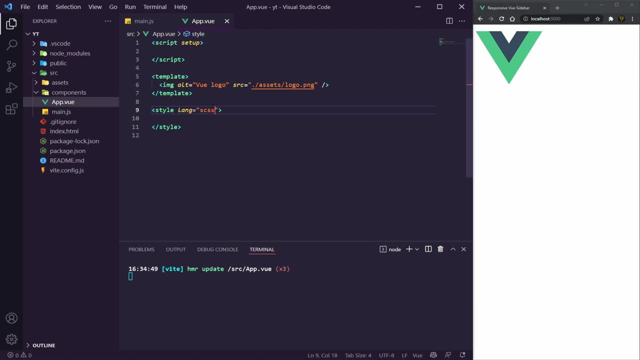 to give this the lang attribute of sas, c, s, c, s, s, which is the language i'm going to be using, and that's why we need the sas installed in our dev dependencies and this will automatically know to use that instead of the normal css. another thing we want to do is inside of our source, we're going: 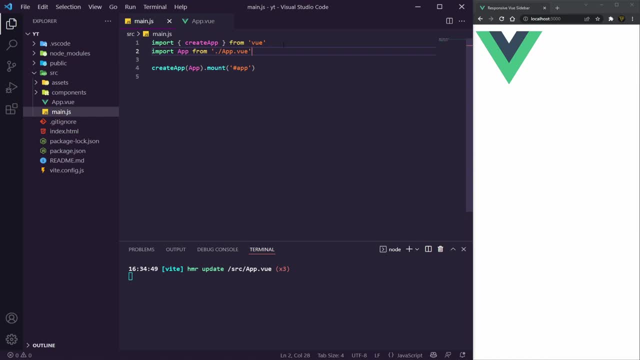 to actually in our main. i'm going to show you how you do it in your main and then i'm going to show you how you abstract this from your main. so we're going to set up our router now so we can route to different pages. one of the things we need is a new folder called fuse, and inside that we need 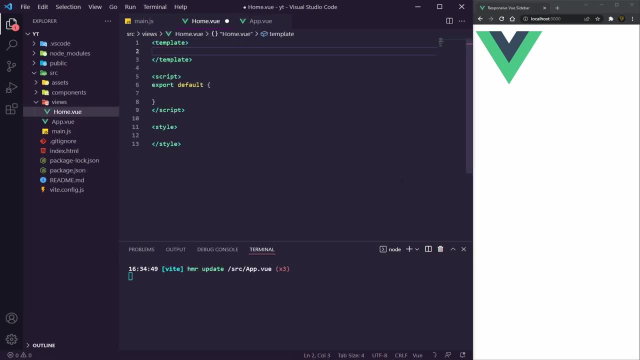 a homevue directory and we could just use basic boilerplate right here. for now. we can give it a main: hello. we don't want. you, excuse me, go away, we just want there, we go, we want a main tag and i'm just going to give it the class of home. 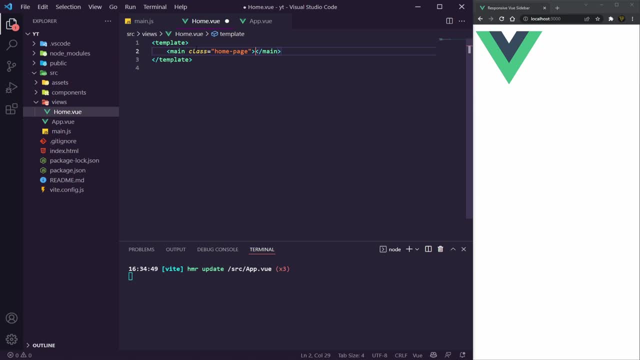 not gnome home page, just like that: a h1 which says home and then, oh said, a paragraph tag underneath saying this is the home page save, and we're going to use that layer. we're also just going to duplicate this, basically, so i'm just going to copy this: create a new, not a new folder, a new file and. 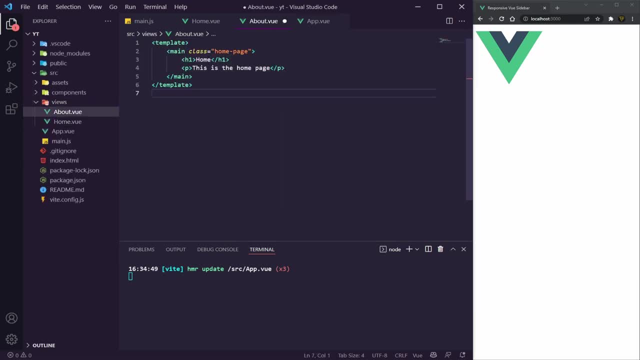 we're going to call it aboutvue and then in here we're going to paste this in. we're going to change this to about. this is going to say about, and finally, this is going to say about page. and there you go. so that's all set up, with some different pages we're going to use and 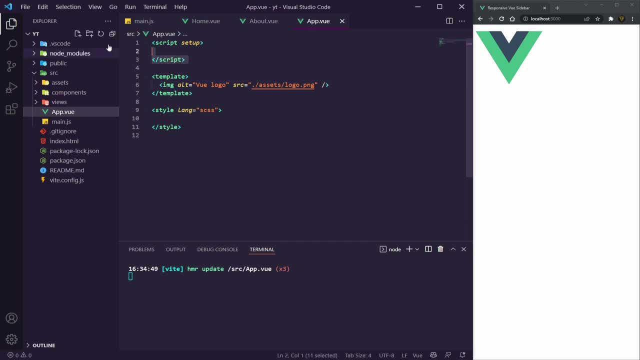 then this route element is going to be where we set up all our route stuff. so i'm going to delete this set tag for now i'm going to keep these two in here, and in here we're just going to delete this. put a div with the class of app on it, just so we can target it, and then i'm just going to do here. 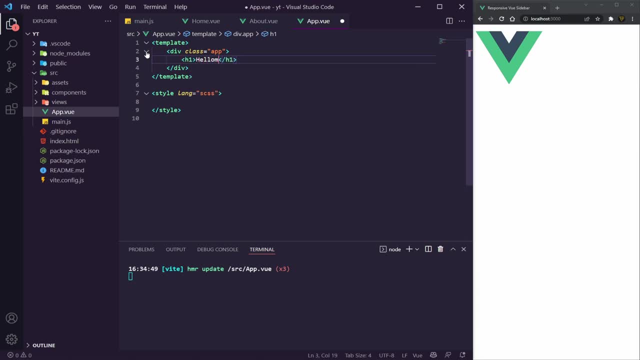 say, oh, just h1 for now. and say, hello world, just like that, hit save and that's changed on the right. there we go now back in our mainjs. i'm going to import in here, i'm going to do it all under here. we're going to say: 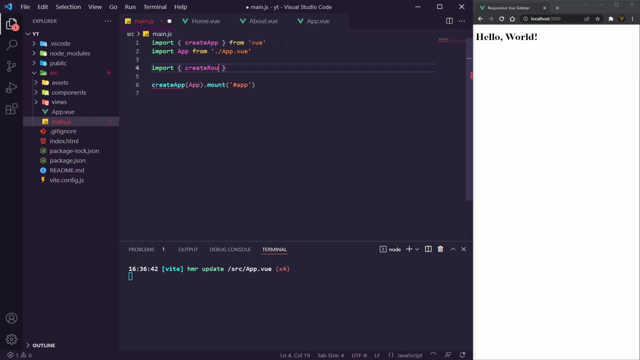 import and i'm going to say: create router from view, hyphen router, just like that. and we also want to get create history as well. so create web history, because we're going to use that to basically make sure we well read it there. create a hml5 history: most common history for a single. 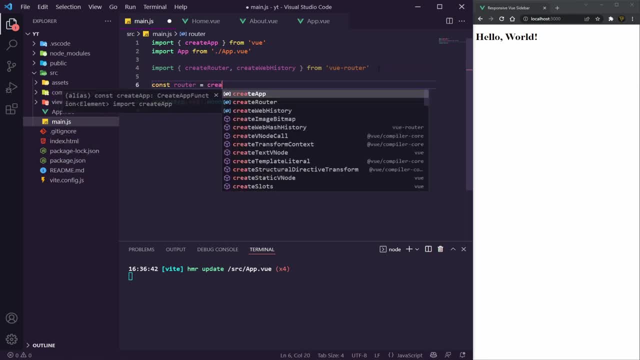 page application. const router is equal to create routerjs. const router is equal to create routerjs outer. and then here we're going to have this and we're going to say history and we're going to set that to create web history, and that's what we need to do. then under here we could have our routes. 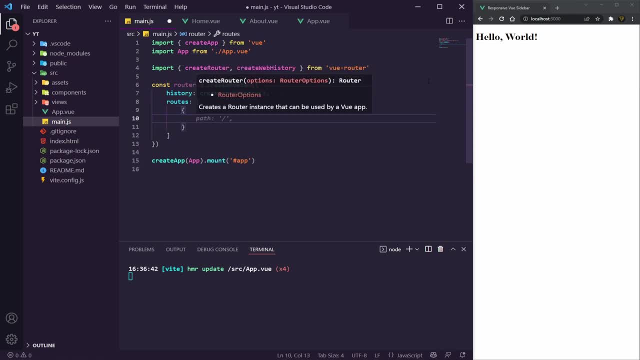 which is going to be an array of objects and we could have some different things. so we're going to have a path of forward slash home or just forward slash, which is going to be our home one, and we could say our component. we could lazy load this or we could import. so let's just import up. 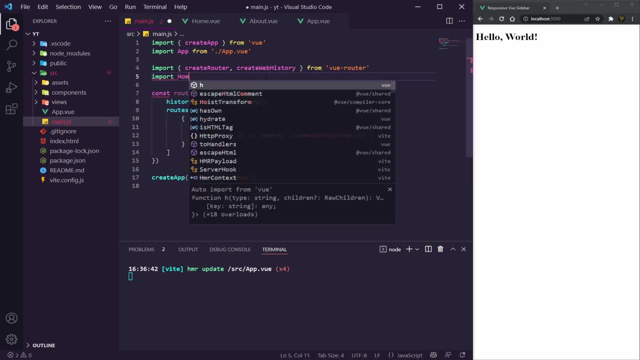 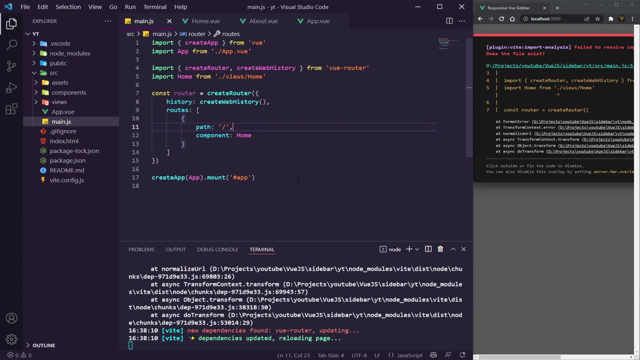 here. let's say import home from, and i could just say, uh, dot slash, fuse slash home, dot view. or i'm pretty sure you could just do home like that. copy this and replace that there, and that will also work as well. uh, what's the sound here? dot home. are we in the? we're in the right directory, right? 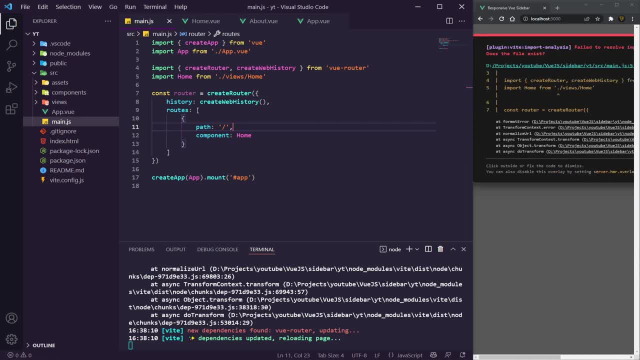 uh, this is how we can't find it. does this file exist? it does, yeah, look, it really does. look. let me just show you. did i name this right? oh cool, we do need the dot view. uh, i don't know why. i think there might be a fight thing, i think. 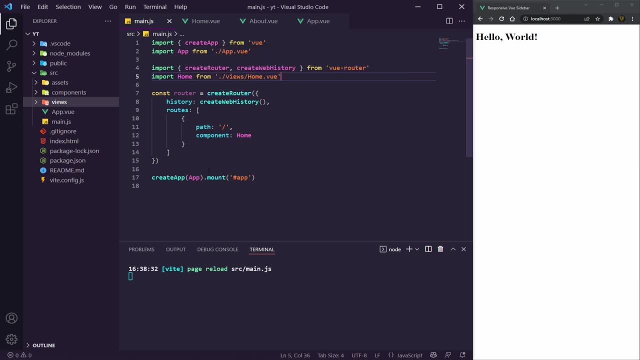 in few, you don't, um, but we bet we learn, we learn something new. and there we go, and then we're going to create a path called about uh, and then we're going to lazy load- excuse me, go away, we don't want you. we're going to then lazy load our about dot view here as well. just like that hit. 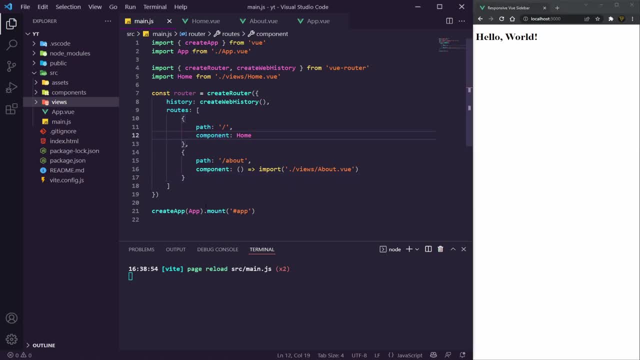 save um and now nothing's going to happen because we haven't set anything up. so we should to actually start using router by doing after the create app: we want to say dot, use router, then mount it to the app like that and that's now going to be using it. but we need a router view in our 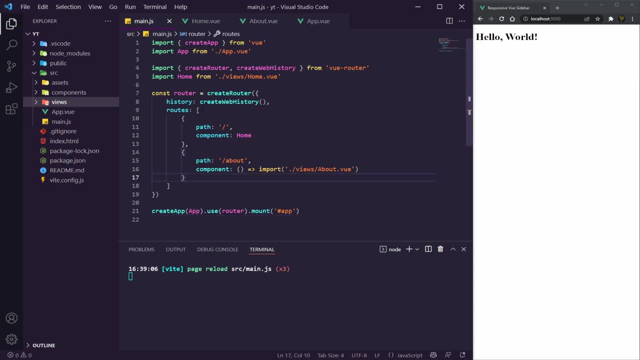 um, main app element here. so to do that, we're going to go down to app um, we're going to delete this hello world and we're just going to say router, hyphen, view, um. and actually we don't even need that, we just need, like that, save and you can see it now. says: this is the home page: um placed right. 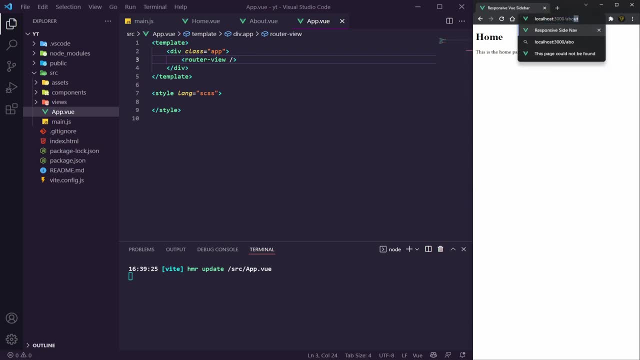 here, which is pretty awesome, and if we now go up here and say forward slash about, you can say it says about: this is the about page. let's go back refresh, because that went back to a previous cached version and here you are. so that is now set up and we're going to have our sidebar above this. 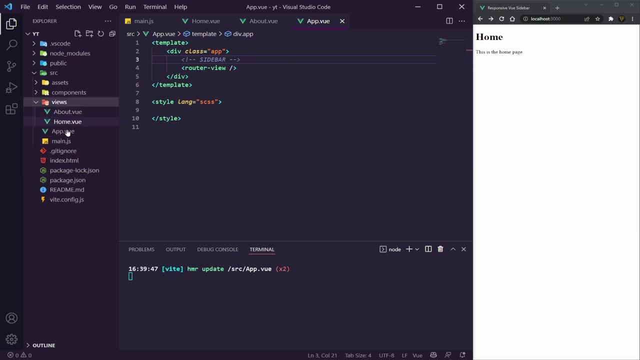 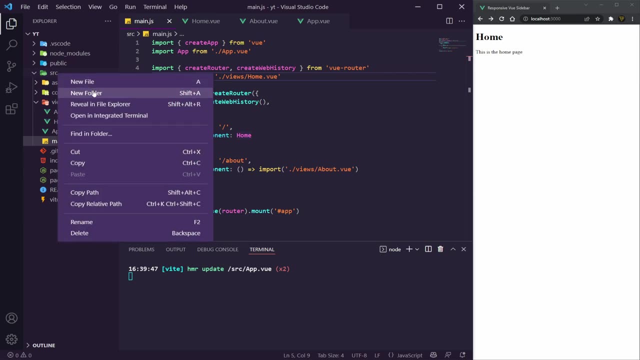 here, um, which again i'm going to go over in a moment. but i want to show you how you could abstract the few routers that we're going to be using to create a router view. so we're going to go into router from inside here to its own file, so to make it a bit near, so we'll create a folder. 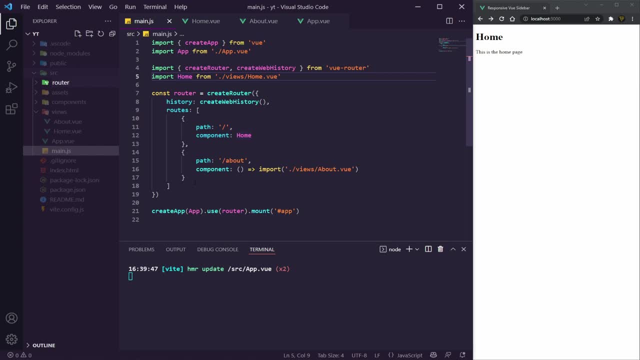 again, if you're building a page which only has like two or three, four or five, just a couple of routes, nothing much to it. doing it like this is perfectly fine. you can do it in the mainjs. it means you don't have to create a whole another folder file or anything like that. but in case, 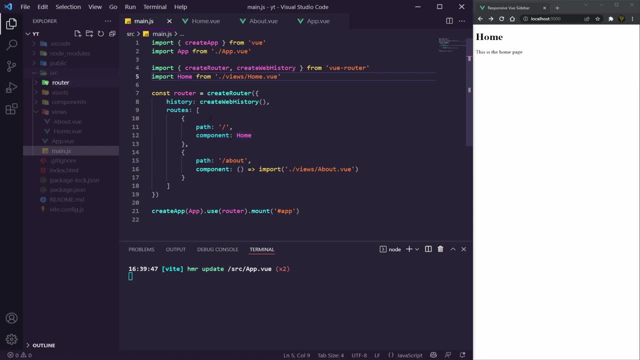 you're building a big app and you need to abstract it to keep it clean, then i'm going to show you how to do that anyway. so we'll go into router and we're going to create a file in here and i'm going to call it index. 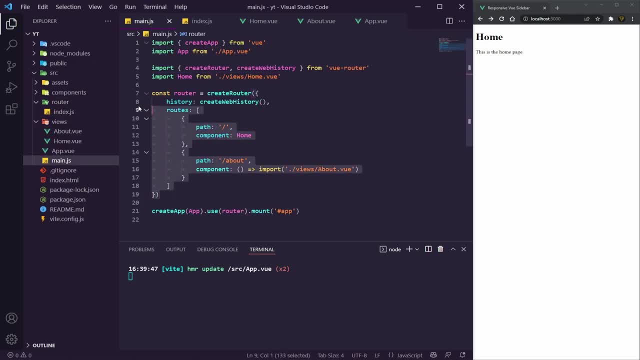 dot js, um, and then we're just going to cut all of this from there, go up here, um, and we'll come back to the main file and we're going to paste it in here. now we need to do so, okay, because this is now no longer true. we need to go dot dot, which means go back a directory out of router. 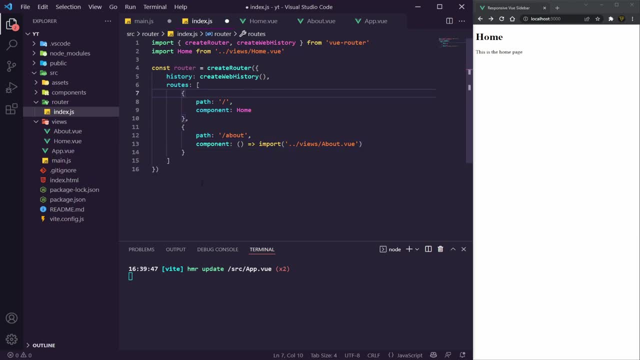 into fuse, and it's the same for this one here, um, and then we need to say export default, and i'm going to say router. so what we're doing in here, let me explain. we don't need that. we don't need that. we're going to have a create router. we're going to import the things we need to create. 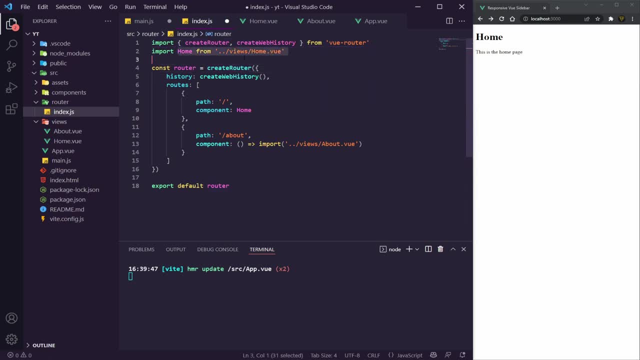 route from few route and create web history. we're not going to create a new one. we're going to import our home view and then we're going to go to our right. we're going to create a new router, um, and then what we're going to do is say the history mode is going to be: create web history. 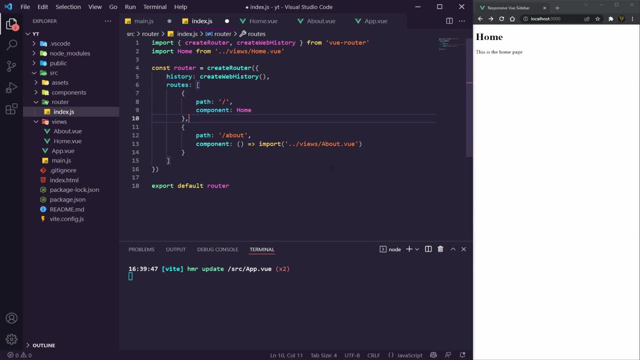 and then we're going to find all our routes in here with a path and a component. now you can do more in this, uh, but i suggest looking at a few router documentation if you want to add like metadata to this. add some other stuff as well, like titles and what else like met, all the, all the. 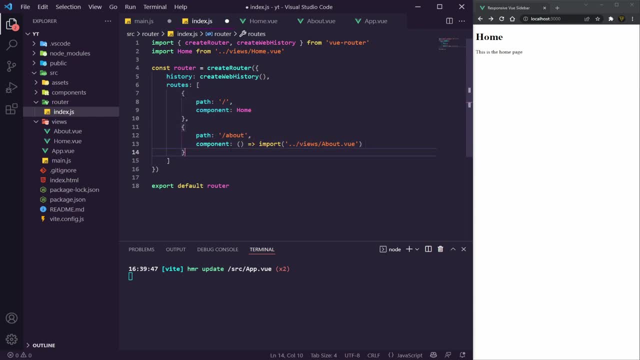 stuff. you could do that in here as well. i'm not going to show you for this video, but if you do want to learn about that, then let me know and i'll do a big, comprehensive, few router video in the future- future, not future- and then we're going to use export default router which is going to export. 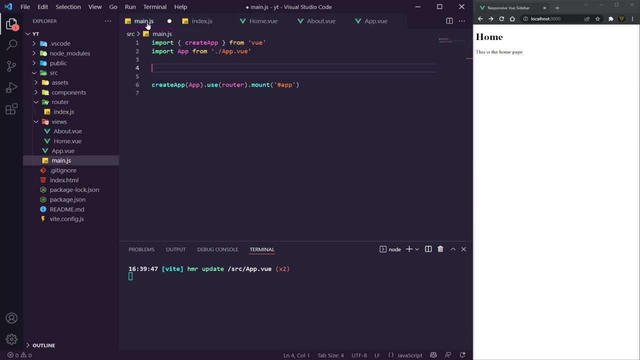 our router component here we've just created. we can hit save and then we can import it in somewhere like this, so we can say: export router from dot slash router and now this will still work as it did. we refresh. we can then go to: uh, we can go to. the next thing we're going to do is we're going to. 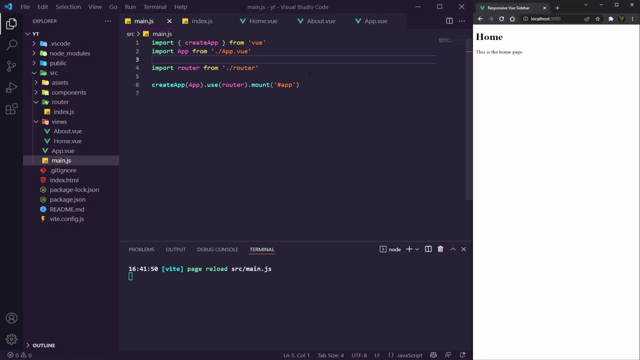 go to about and you can see it's all working perfectly. and there you go. so that is that setup, ready to go. few router is installed. we're all excited, you're excited, i'm excited, i'm hyper, by the way, if you couldn't tell. so that's where we're at, so we can close that file now. we can even close. 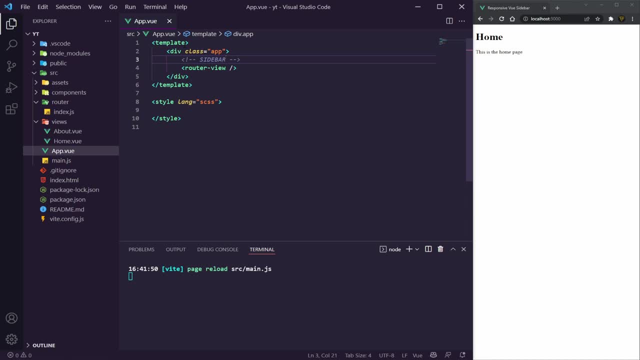 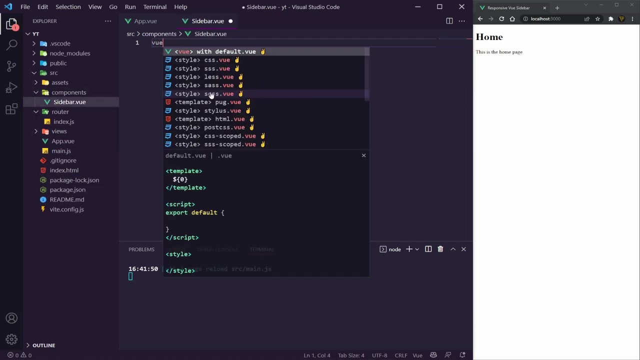 the home and about folks. we're not actually here to learn about the pages. we're here to make a really awesome sidebar in few js. so we're going to create a component for this sidebar. so in here i'm going to say sidebar dot, view and i'm going to run few. now you might be wondering: wait a second. 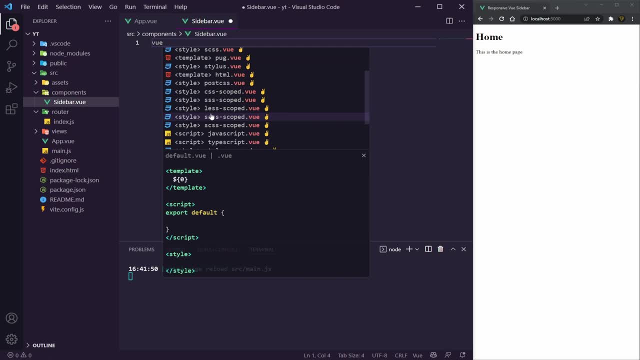 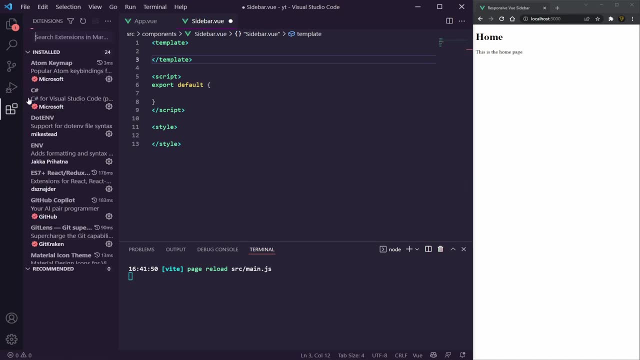 tyler, you just type few and you've got the option to view with default and all this other stuff here. so if i hit any, you can see create a template and you'll be like: whoa, that's a lot of code. how did you just do that? well, i have an extension called future, um, or future future by pine woo right here. 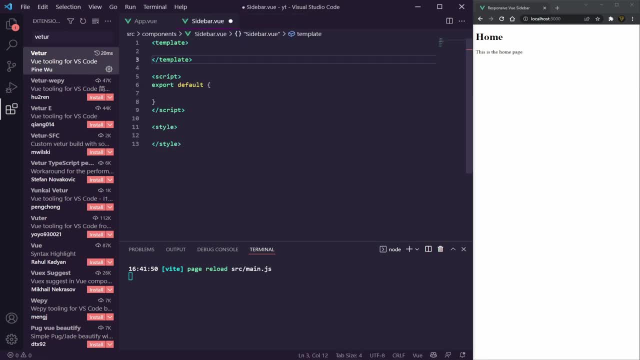 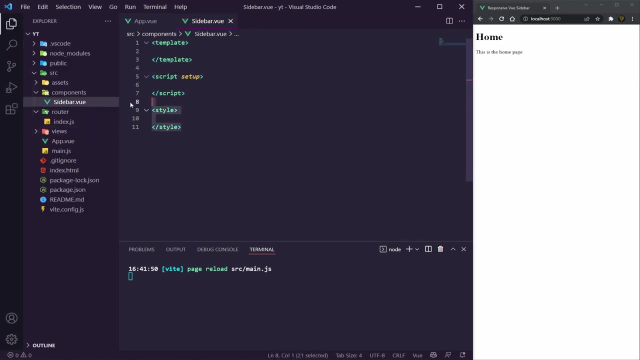 this one, install it. it gives you all the features like this to be able to quickly template an app. so if you're using a few two options api, we can easily update this to say setup. just like that, hit save and that's now using the updated version, we can go in here and if we want to, we can delete this. 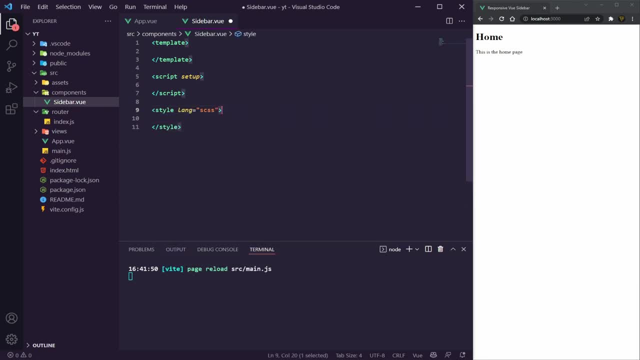 and just say sas, like that, and hit sas. we can also pass the scoped attribute to this. um, or is it scope scoped? you know what? let me show you. this will also tell us if we go style, look for the sas scoped, or sc, TSS, scoped. and there you go. That's how it sets up. So it's super simple, gives you a bunch of awesome tools and 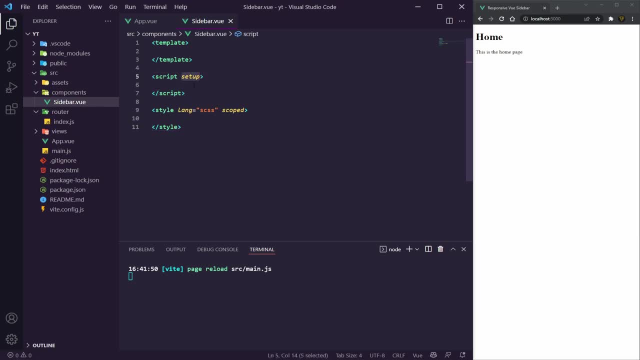 Hopefully they update it soon to have This setup as a default thing you can initiate, instead of because you can do. if you type in script, You can see there's a bunch you can do with like Yeah, well, there you go. Look, a bunch of different things here. 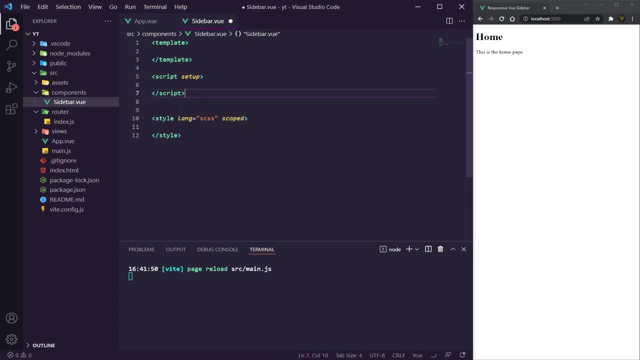 I have to do to do different types. That's type scripts. You can do it with whatever else, but there you go. So that's what we've got set up, and now in here We are just gonna write a site which is the sidebar tag, Which the HTML, HTML semantics there for you, and then let's just do a quick test and it's a sidebar like that. 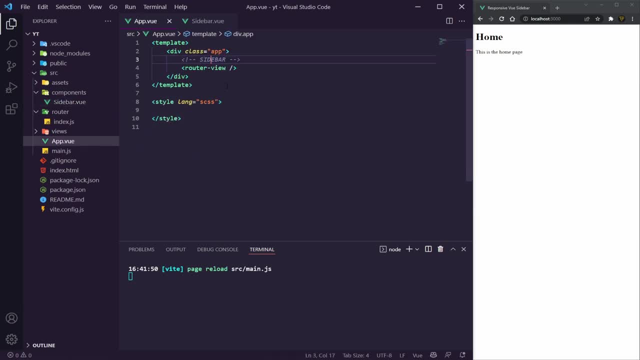 Hit save. we'll leave these blank for now. go back into our app and now we need a script type. So I'm just gonna create a JavaScript script tag, I'm gonna pass setup in here and, for those who use the options API, Well, this just basically does a bunch of things for us. 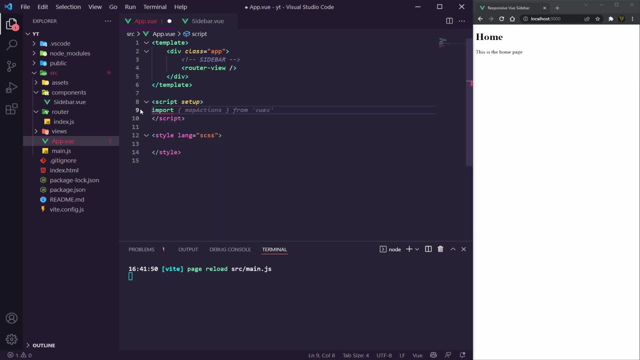 So in here we can sue something like import and we can say side bar From and we can just say dot, slash components, slide bar, not cider bar, just side bar. and This, how simple it is. You don't have to explore it in few options, You have to return it inside off. 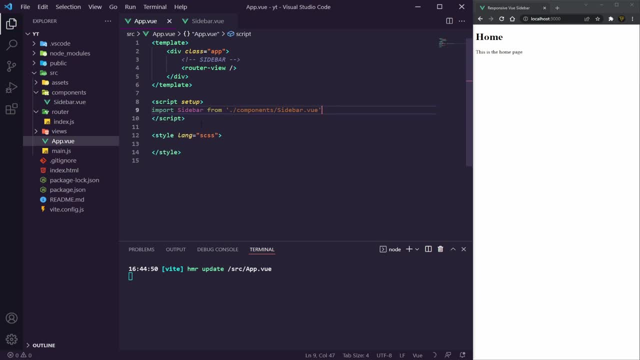 Well, even inside of the setup API- composition API- you have to return it. However, in this we just have To type it like this side bar And there you go. You can see it's now employed at the top here, which is absolutely awesome. 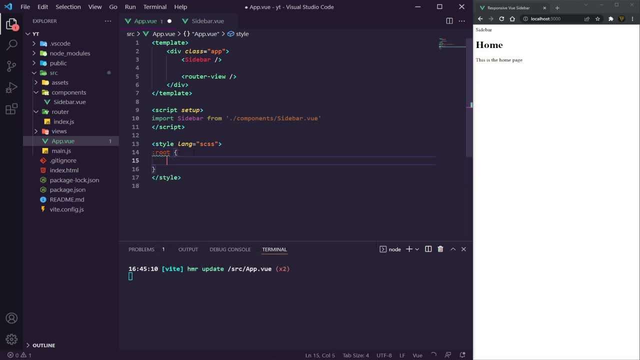 I want to do a couple of things. to start with, I'm gonna create a root element here. I'm actually gonna copy some code For my actual colors. So inside of our style I'm just gonna paste in a bit of code. I'm gonna close this. 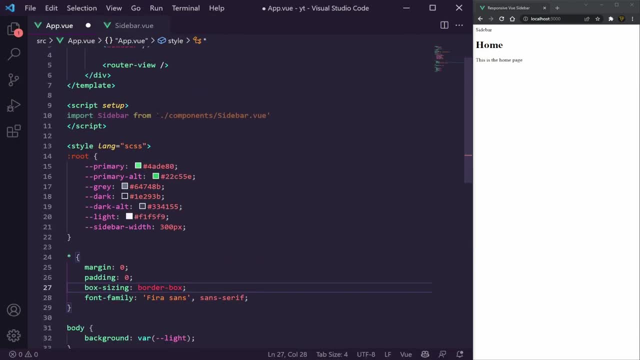 I'm gonna minimize your sidebar and I'm gonna zoom in one as well to make it easier for you to read. hit save and you Can see everything's sold up a little bit. but let me explain what CSS I've just added in. so I've added in this root element here which could allow us to define some roots. So document level: 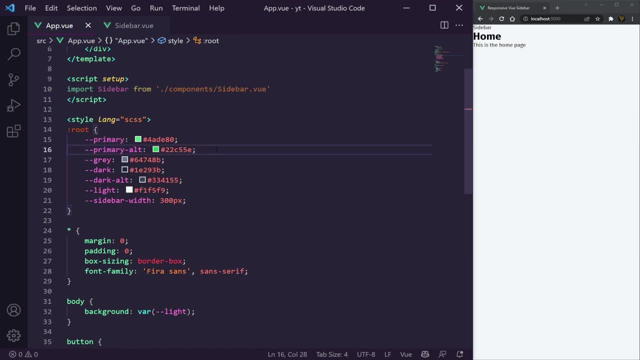 Variable. so you see, we've got primary, primary, Oh, we don't actually use that, so I can remove that. We've got gray, dark and dark, Oh, light and the side bomb. what? that's a max width, But we could also add a min width as well, But for now I'm just gonna do sidebar width. 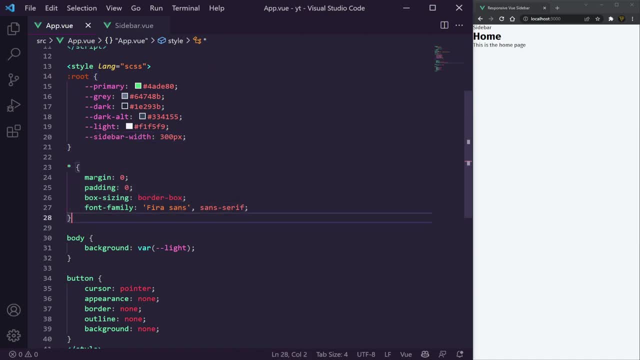 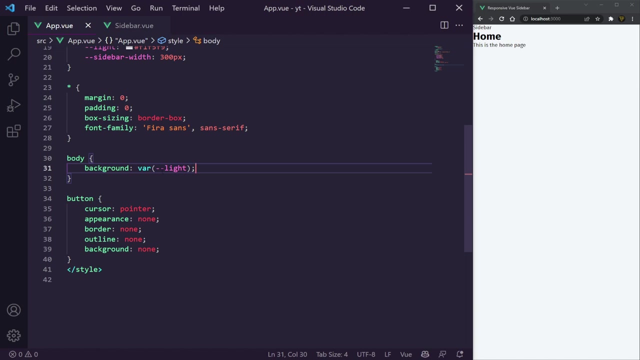 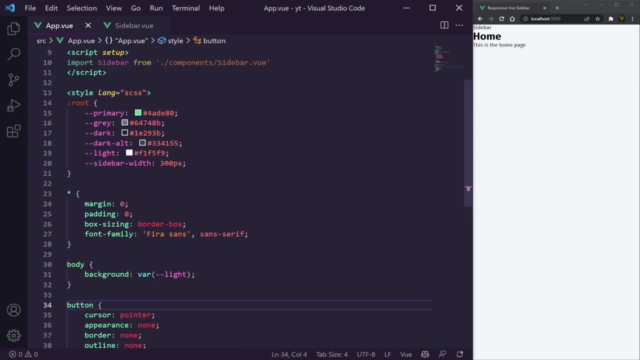 Hit save and that's that. I then added in some resets to remove all margin of elements, All padding, any box sizing, and also added the fire sands font which we imported earlier on in Google fonts. I then added a lighter color to our body background by adding far, and then I've reset buttons to basically have no styling to start with, so they don't look weird when. 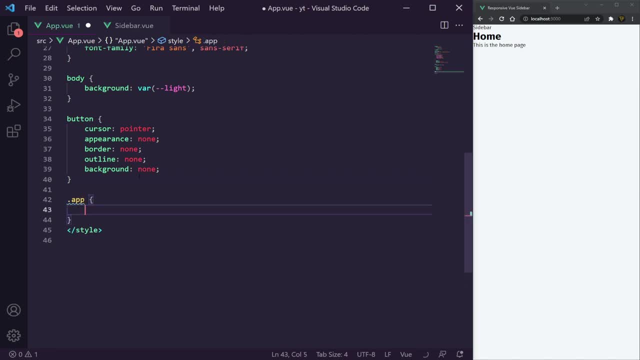 We start styling them and we're gonna have one more thing: We need app and we're gonna have to display this as flex, which puts them side by side, as you can see, which is really nice. We can then go in here and we don't need to flex direction column. 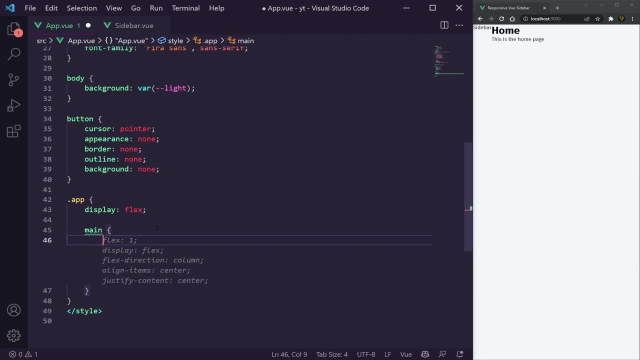 We can actually just say main, and the main is gonna allow us to say: flex one, one zero, Which will stretch that out to be as big as it can be. We're gonna set some default padding of two rep. We're just gonna push it out a little bit and then, because we're actually going to have this sidebar on, 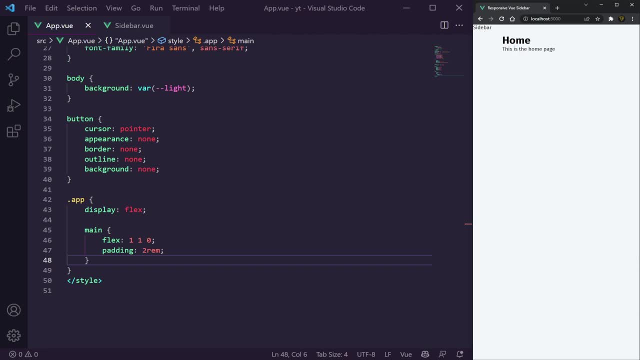 Mobile be an absolute element which sits on top. We're basically going to just remove This. well, this is actually gonna end up seeing right to the left, So we need to do so here. when you say app media max width 768 pixels, so on iPad and below, we want to set the padding to be six REM, like this here: 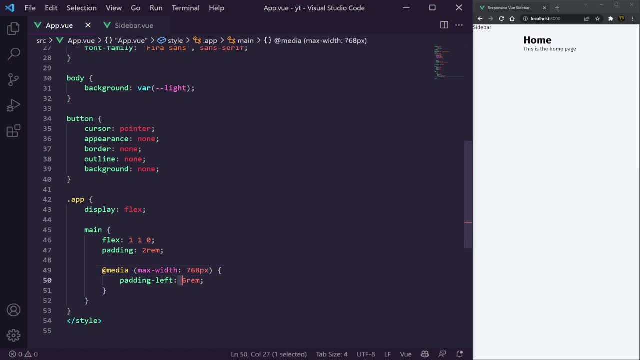 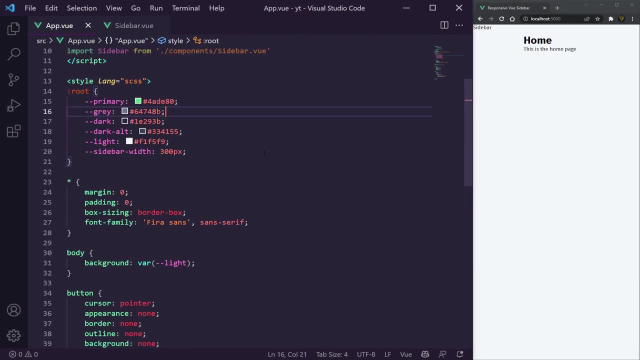 So you've got the 768 and padding around there. So here you go. So you can see that's really far over and the sidebar is just looking a bit weird. So that's all we need for this app dot view. by the way This is now doing, we can actually close. 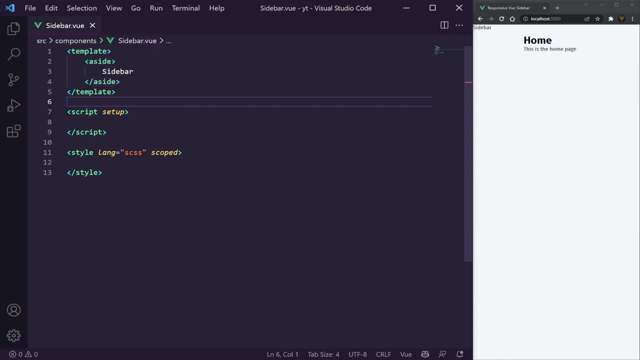 this app. Everything else could be doing is practically inside of sidebar dot view, So we're going to start off with styling this inside of here, because it's scoped. We don't have to worry about writing something here, That's gonna style something else. It's only gonna style this stuff inside a template, which is great. 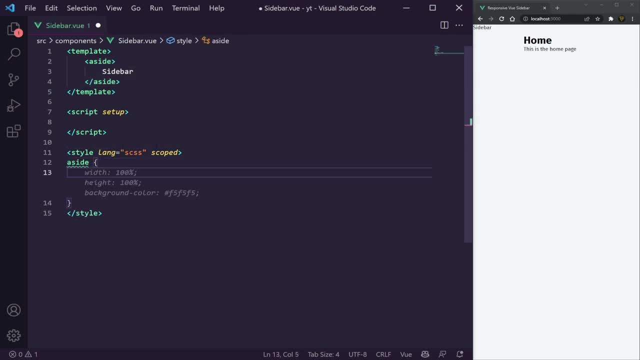 So we could just say a side like this without having to give it a class, Although a class would help. this is just simple. We're display this as flex and we're gonna give it a flex collection of columns. You want anything to go down? We then just want to say: background. 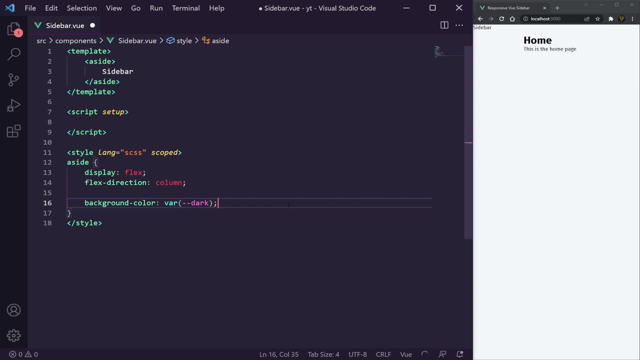 Color, it's gonna be equal to one of our variables, which is gonna be dark. so if we just say, if you can see, that's now dark, we don't want to add in a Color as well, a far light, anything in it, All the text will be a white color, or you could just do white here by saying FFF. 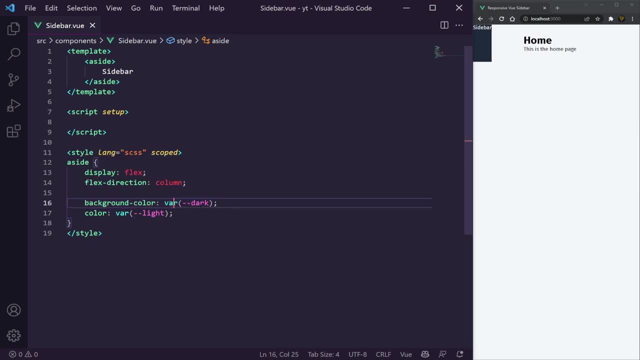 But I just prefer to add in a slightly dimmer color so it doesn't hurt your eyes. and then I'm just going back up here. I'm gonna say: width is equal to far sidebar width, which you're gonna see. It's push out 300 and you set overflow to hidden. 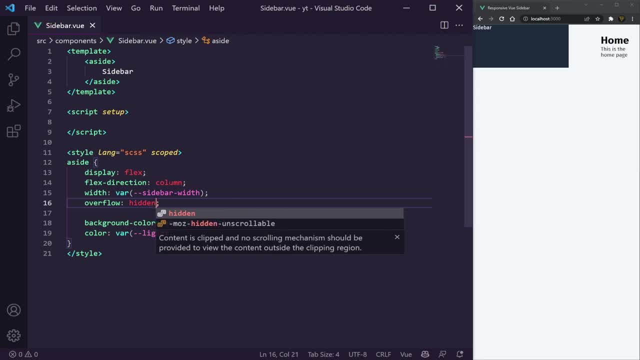 so if it goes off screen, it all gets hidden, which also gonna help out with. there's a key element that helps us with the Sidebar shrinking and growing. we want to set a min height here to be- let's bring this up- a hundred VH. That's just gonna make it the same size, our screen. 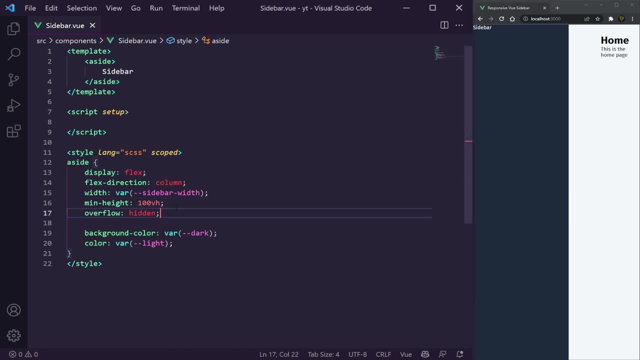 so it takes up all the space we require it to, and We're just gonna add a padding of one rem, which is equivalent to 16 pixels right now. finally, At the bottom, I'm just gonna add a transition of 0.4. like that I'll 0.2, even to make it a bit quicker and say ease. 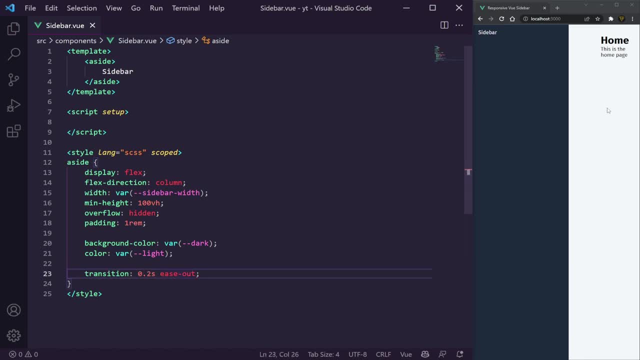 Out, which can allow it to when we actually do the transition of this opening and closing. It's gonna basically slide in and out, which will be nice. So we're not gonna do a media query in here And I'm just gonna say media query, max width of seven, six, eight pixels and we're just gonna say position. 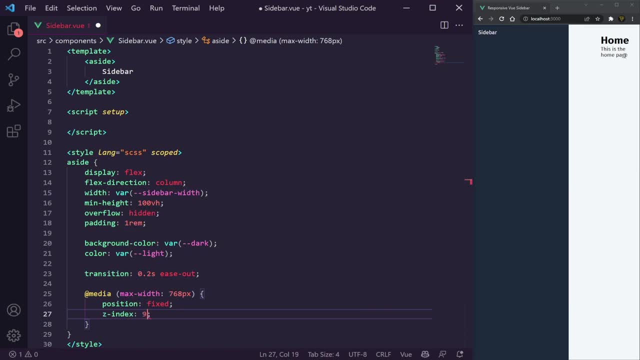 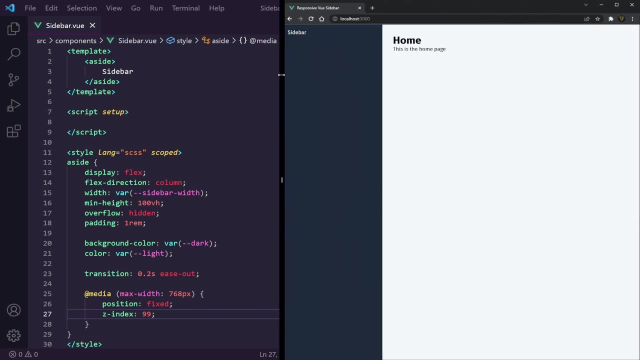 fixed. and then we're gonna say: See index 99 to make sure it's on top. and there you go. You could now see that's hidden, the elements are gone And if we stretch this out, you can see the homepage reappears. to reason: the home page has disappeared. 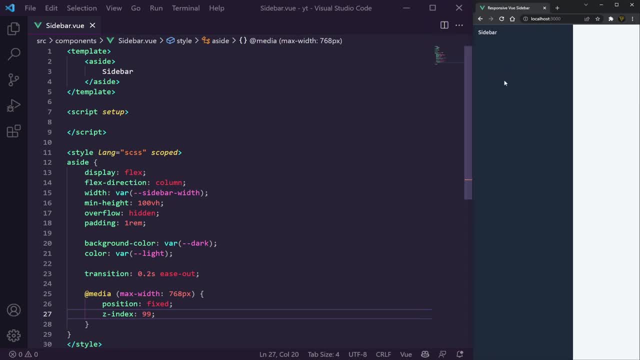 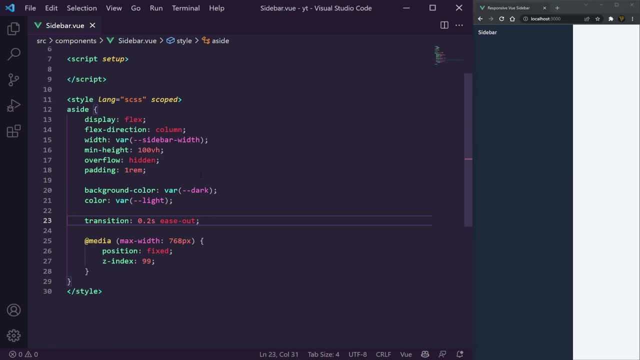 It's because actually got behind this bars. if we was to delete this bar, the inspector Delete. you can see home is still there. It's just underneath it. We're actually gonna have this closed by default, so we can see that. so let's go in here. 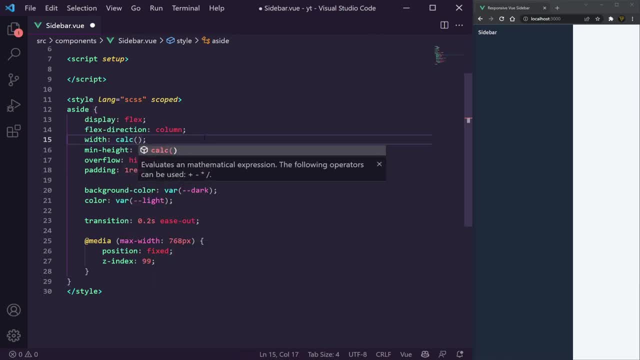 And we're just gonna change this from being fast to count Because we're going to calculate, we're going to use some maths here to do some things. Let me show you. We're going to say calc 2rem, which is double our padding on the left and right. 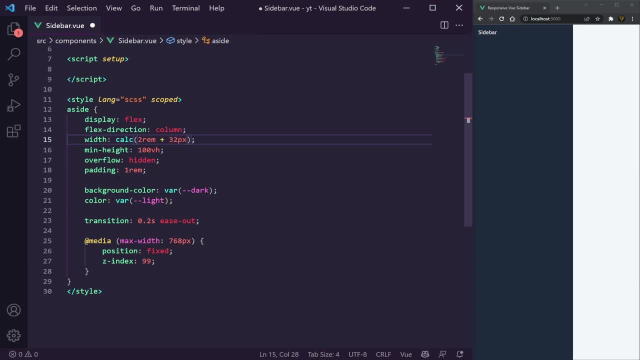 Because we need to do that Plus 32 pixels. Now, the reason we're doing plus 32 is that's how big our icons are going to be. So we're going to have our icon size plus the padding on either side, And that's going to give us the width of our sidebar. 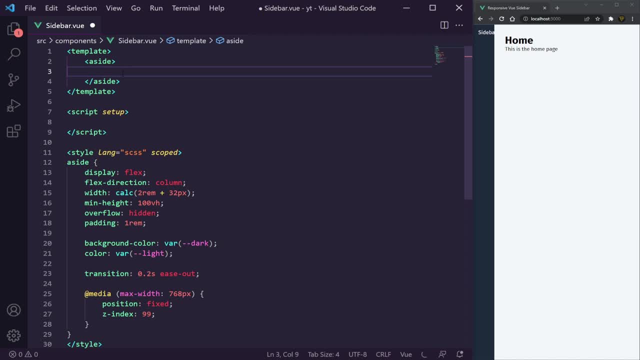 And there you go. That's that there. Let's go up here and just remove this for now And we will add in the logo as a placeholder for now. So I'm just going to say dot logo, I'm going to say image. 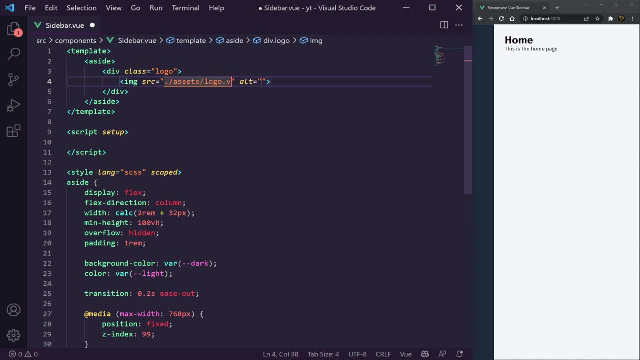 We're going to say dot slash assets slash logo, dot png. It's a png, not anything else, And we'll just say view in there. Oh, and that's not loaded. That's because I have done it wrong. It should be dot dot slash logo, because we're currently in the components directory. 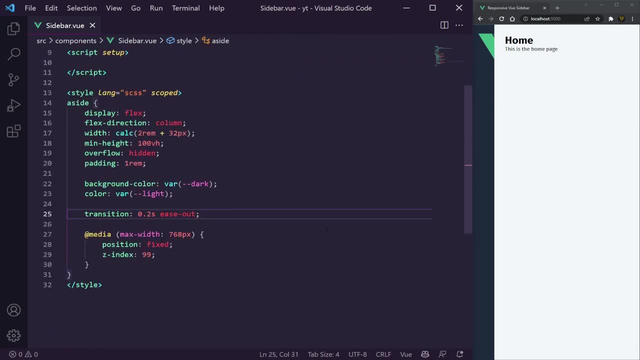 And you can see that. that's there, but it looks a bit ugly. Let's go. So inside of the side tag we just want to say dot logo And we're going to give this a margin bomb of one rep which will push anything inside of it down. 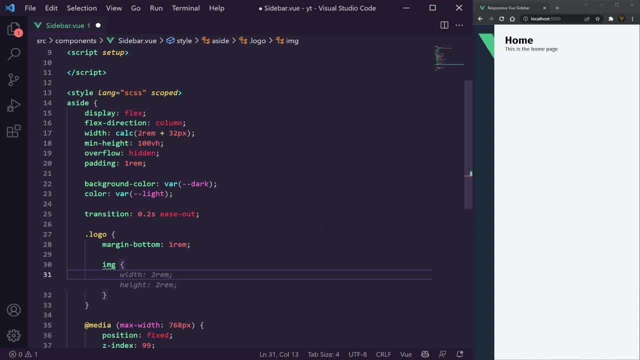 I'll anything below it down, And then we'll add a well, a margin bomb of width to rent, just like that. We don't need the height, And there you go. That now fits in our element. 32 to rent is equal to 32 pixels. 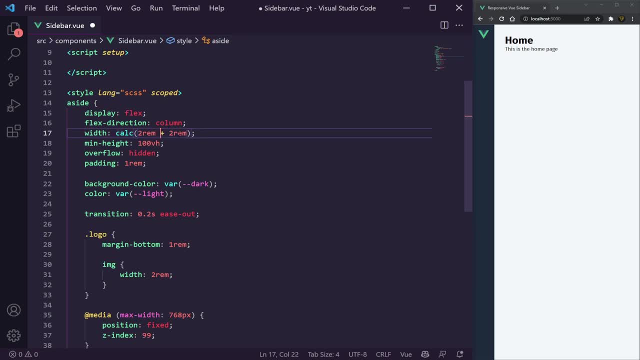 So we can actually change this to two rep, which would also Make sense. I just like using the pixel value here. We could also just say four rem here if we really wanted to, but using the calculations means we could change this into a. 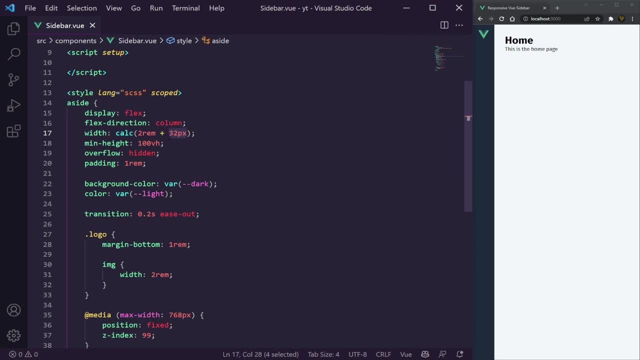 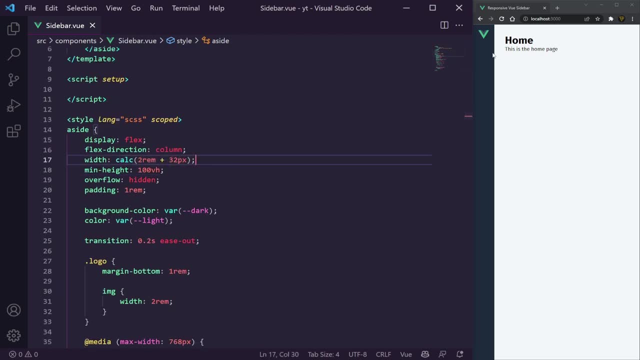 fairy ball and change the width for icons and if you anything else using that there, I'm not going to do that right now, But it just gives you an idea of why I'm doing it like this. And there you go. So now we've got a little side by there. 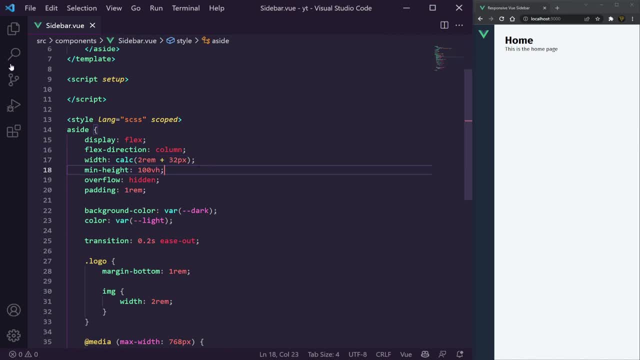 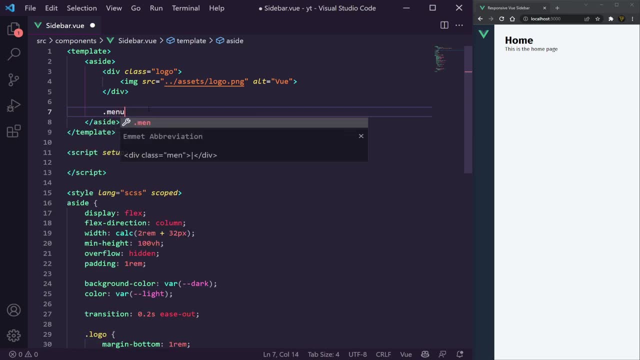 Let's get in the actual icon to open and close the menu. So underneath our logo let's give it a couple of spaces. Um, we're just going to say The uh dot menu toggle wrap. There's going to be the element around our uh menu toggle. 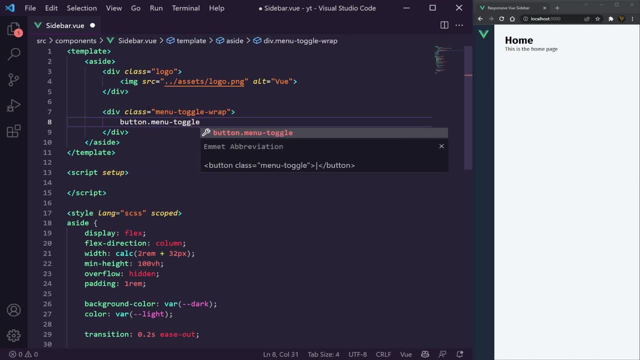 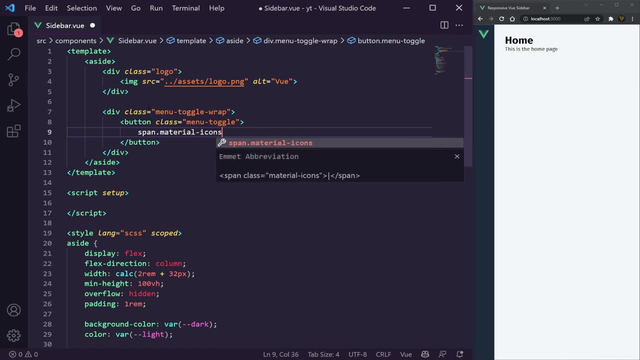 Well, they're going to have a button with the menu toggle class And then inside of here we're going to have a span with the class of material hyphen icons. Now this basically says we're going to use material icons and we need to give the icon name inside of here. 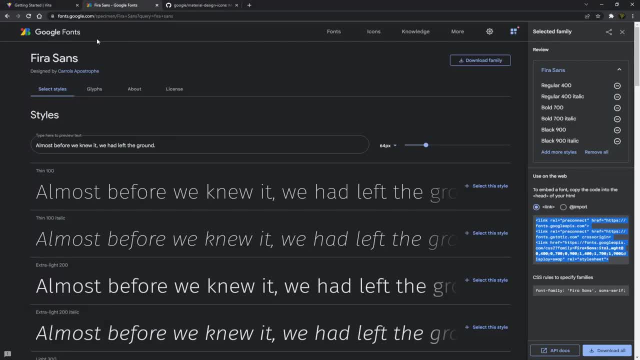 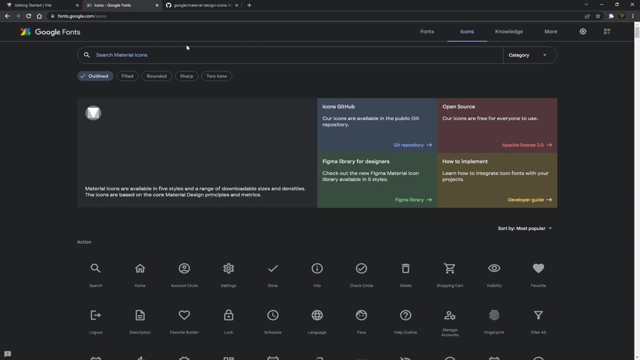 So I'm just going to show you. I know what icon I need to do, but I'm going to go and show you how you get these icons. So if we go to fontsgooglecom, forward slash icons, you come to this page and we're looking for a double chef, Ron, a double arrow chef from this thing here. 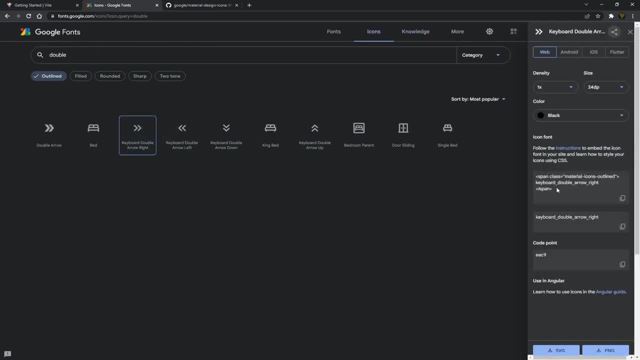 So we want this one here to keyboard double arrows. If we click this, it shows you how you could use it with the span. That's the outline You can see. we could change it to field, rounded, sharp or two tones, but we actually only have the field element installed, because that's the one we added. 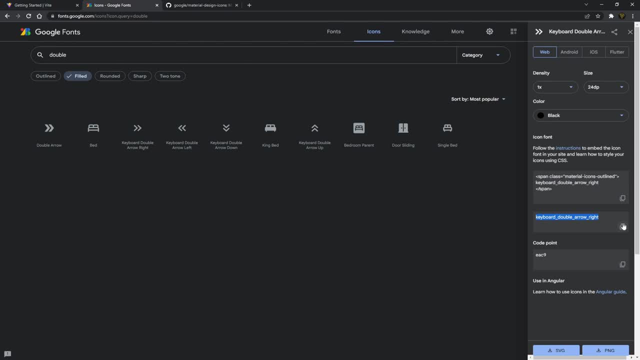 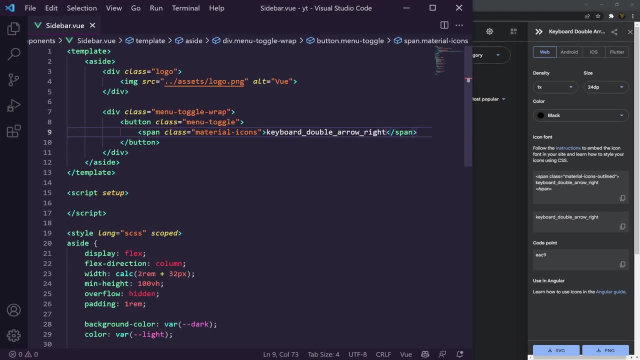 So we're going to use the field and I'm just going to say I'm going to select this text right here. I could copy the whole thing. I'm just going to click this and they're going to go to here and what you're going to paste that inside of here. 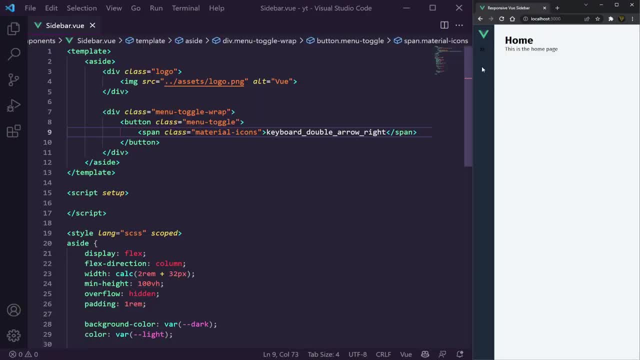 Now, if we will open this up and reopen up this, you can see the icon is actually there. It doesn't look very good, It means styling, but you can see it's there and it's clickable. We could also add in here a click event which we're going to call toggle menu, just like that. 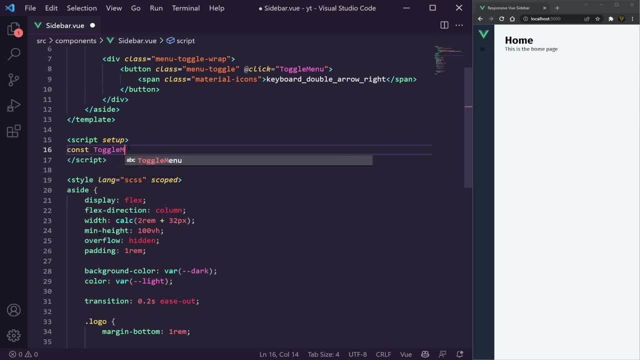 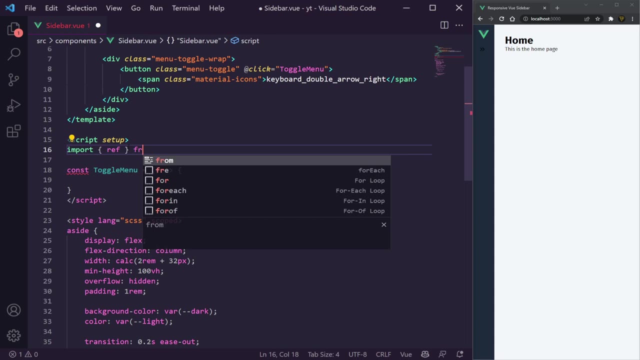 And in our setup we could just say: const toggle menu is equal to, or what It's actually going to be: equal to an arrow function which will toggle our menu. Now we're going to import something from view js, We're going to import ref from view and then we're going to create a new thing called menu open. 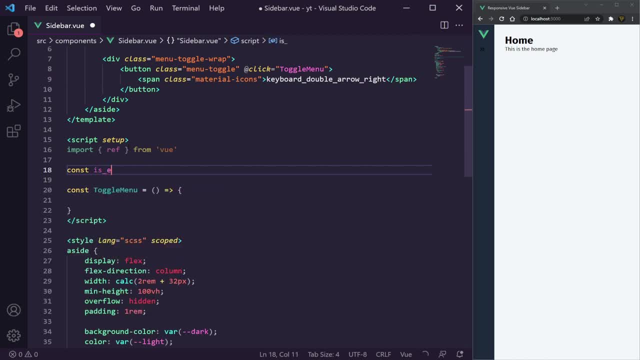 What should we call it? Let's call it expanded. We're going to say: is underscore expanded, which means our sidebar. We're going to set reference To false by default. So now in here we could just say: is expanded. dot value is equal to not is excited. 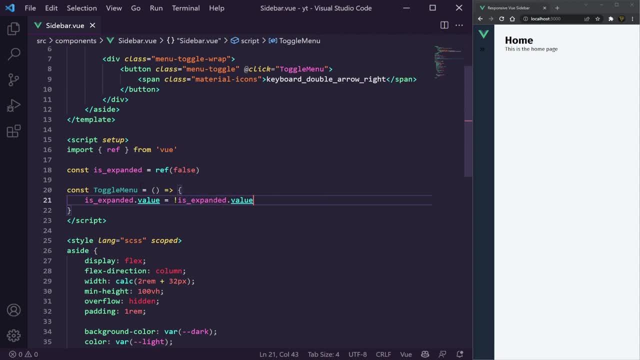 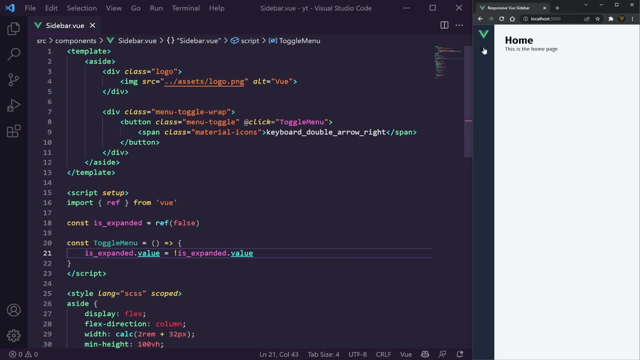 So, whatever it is, sell it to the opposite, and that is all we need to do, And that's not going to be pulled in here, Obviously, if I click it, that does nothing. It's going to change the value, but you can't see anything happening. 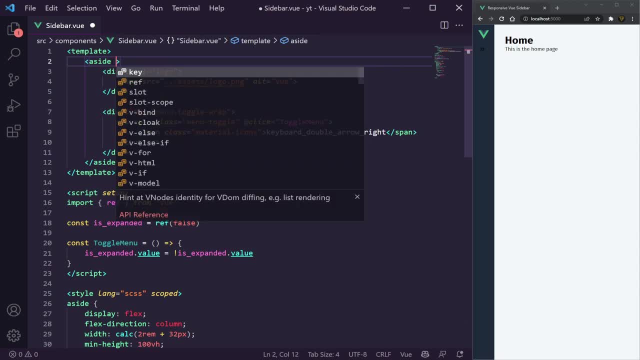 So inside of our side tag at the top here we can actually bind a class element. I'm just going to use back ticks here to be able to use temporary literals. I'm just going to use this and I'm going to say: is expanded. and I can just say: if it's expanded. 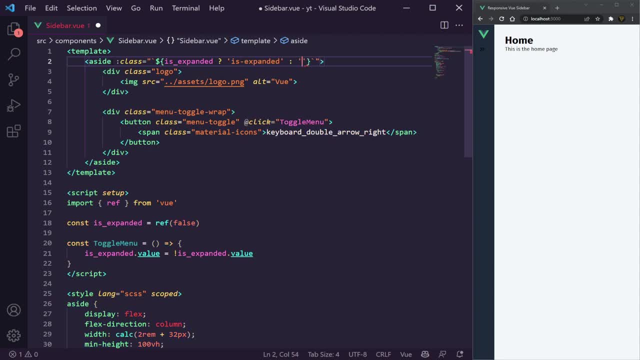 we're going to say is hyphen expanded? Otherwise we're just going to pass through a default empty string there, Hit save And there you go. I believe you could do this shorthand as well by just saying and and like that, and that will basically work as well. 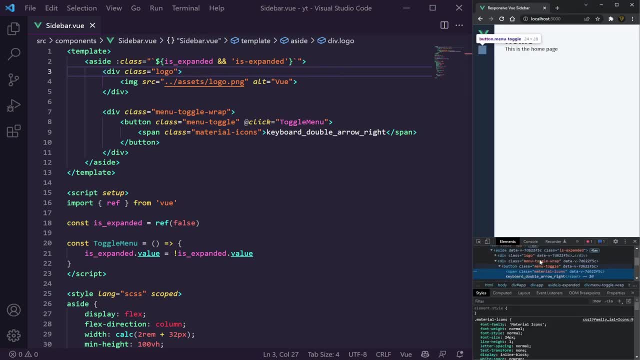 So if you click that and we let's inspect this here, you can see there It says is expand. If we click it again, it removes it and just puts false. Yeah, so it puts false. If you use the other way of doing it, it won't put anything. 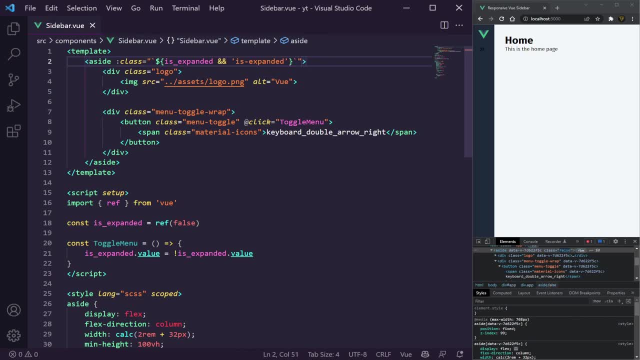 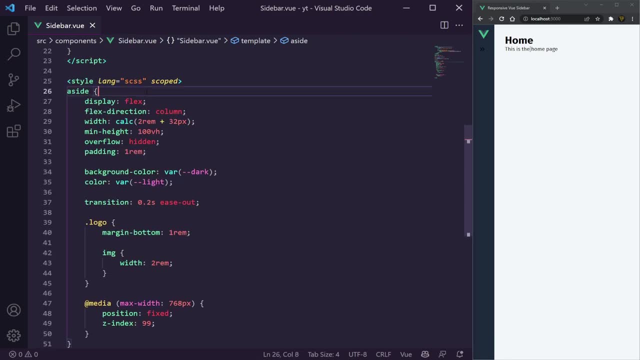 You'll just leave it as empty, but the shorthand looks neater, So we're going to go for that. now, This doesn't do anything because we need to actually add some CSS to get this to work, So let's go underneath our aside here. 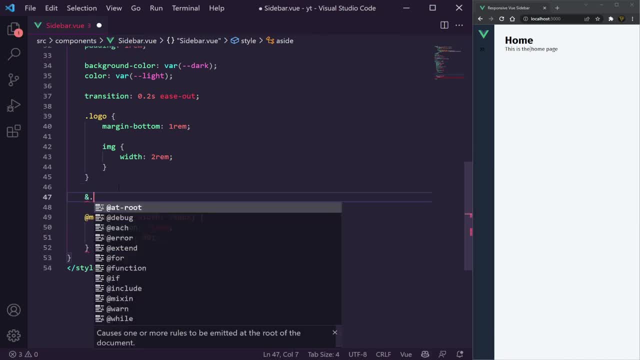 And before the media, let's just put in a and dot is underscore, is hyphen expanded, and then we can add all us, us, Well, all Our styling in here which we need for it. So the first thing we do is really give it its width to be equal to the variable we set, which is sidebar width. 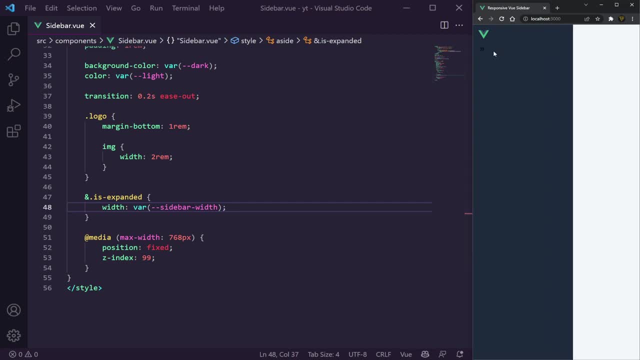 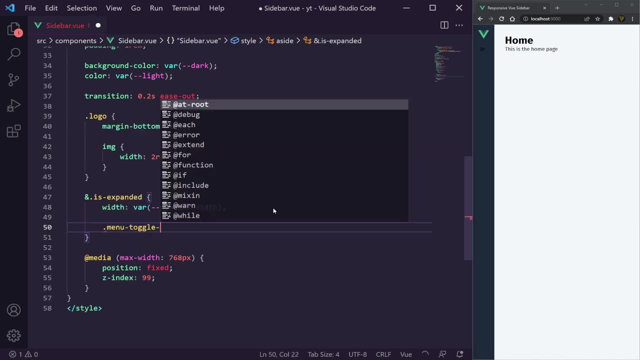 So if we now click this, you can see that expands, And if we click it it closes, which is pretty cool. We then want to also go to our menu, Toggle rap, And we're just going to basically say: top is equal to minus three run. 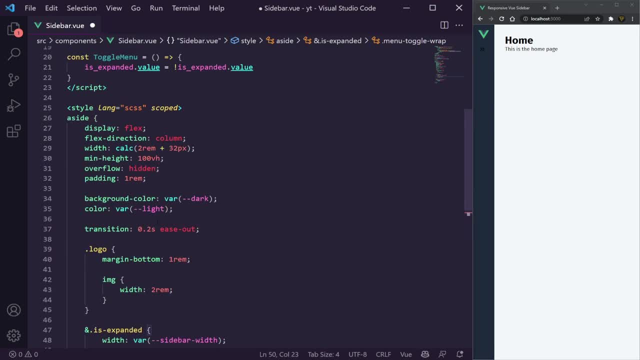 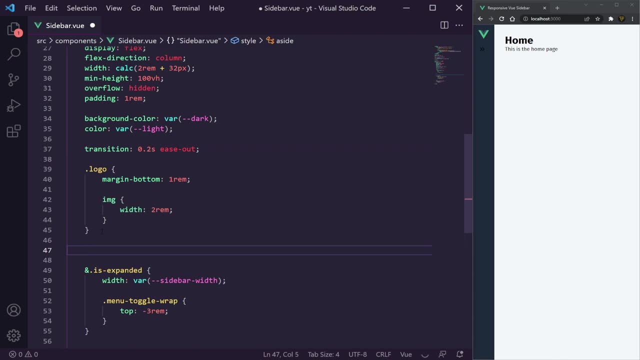 Now, This is a good do anything yet, because we actually have installed this menu toggle wrap At all, Anyway. so let's go back to our side tag. underneath the logo, We're just going to basically add in the menu toggle wrap class. 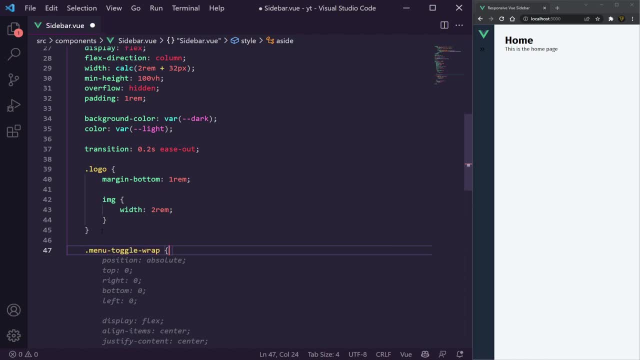 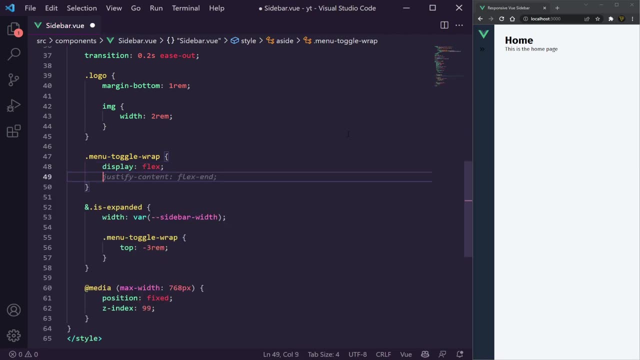 So, just like this dot menu toggle wrap, And in here we can basically add a bit of sign. We can display this as flex for stars. Well, they're going to give it justify content: flex end, which is means it's always going to sit at the end of this element. 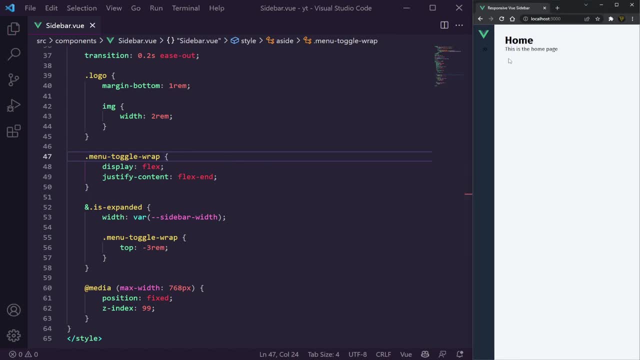 So when we open it it will sit there. Let's save this. You can see. So you can see. it now sits at the end. We can then also give it a margin bomb of one rep, because we're going to have a menu and deal. 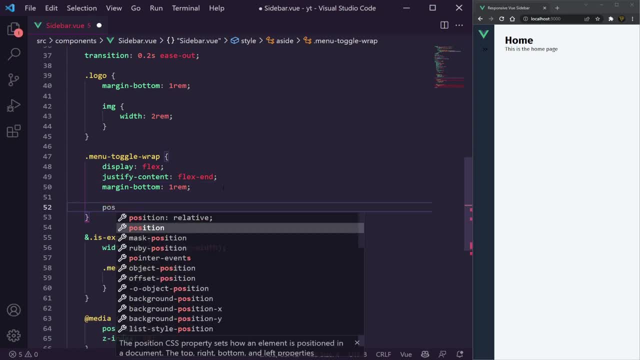 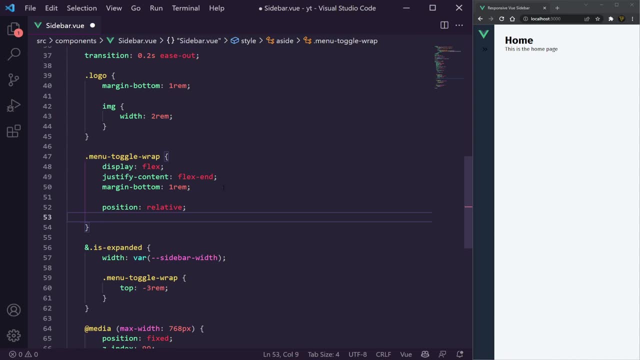 We need to push down. We don't want to set this position equal to relative And once we got the position equal to relative, we can add a top of zero. It's not necessary, but I like to add it there for fish will purposes, and then we can say: transition: 0.2 seconds, ease out like that. 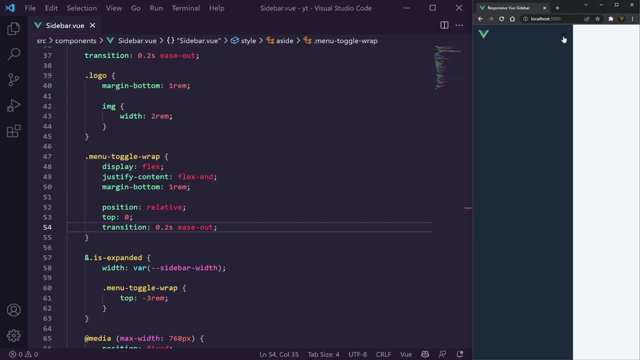 Hit save And now, if you click, you can see that It moves upwards into this gap, which means it's in line, So it no longer sits below this and looks all ugly. It sits next to it because if you just pulled out here it would look a bit weird. 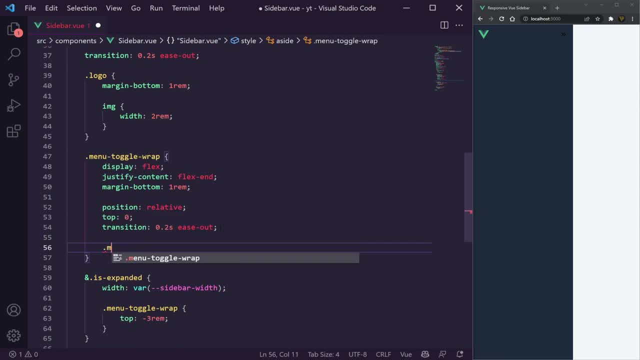 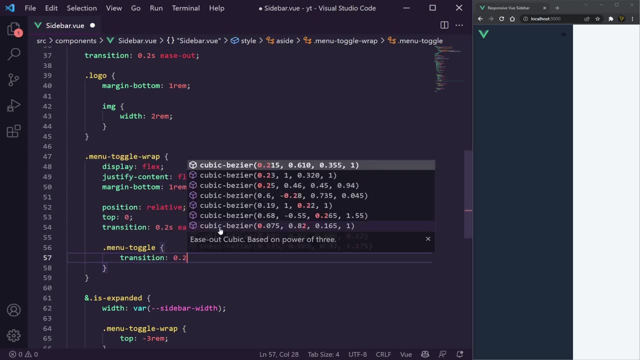 So I brought it up. That's what we did. Let's then go into our menu. I'm from toggle and now in the menu, toggle, we're going to give this a transition of 0.2 seconds: ease in or ease out, like that. 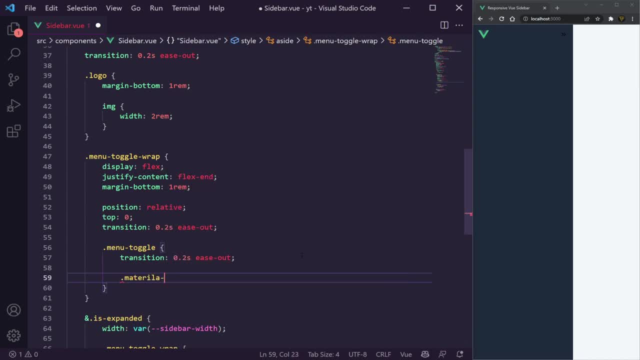 And I'm going to get the material- Well, the material icons, which is the class for our icon here, And we're going to set its color, but we'll say it's fun size to be to rent, which is 32 pixels in this case, and our color to be light. 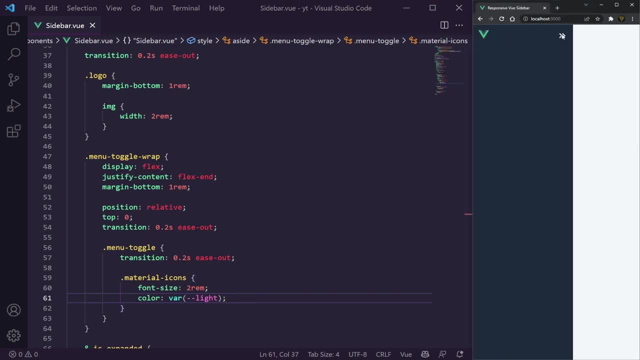 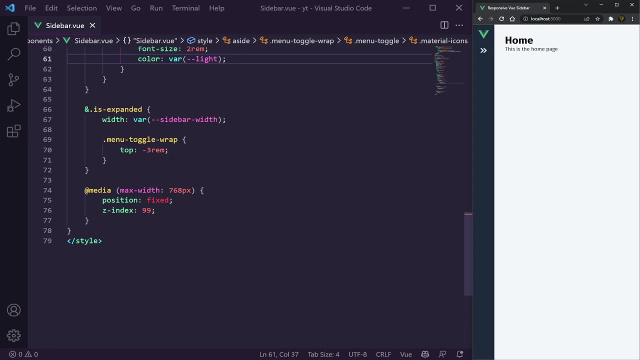 So you can see there. that's now there, But when you have it open you can see it does not. It's facing the wrong way, So we need to add some styling to that which deals with it. So let's go all the way down into here and we'll go to menu hyphen toggle and we're going to pass in a transform. 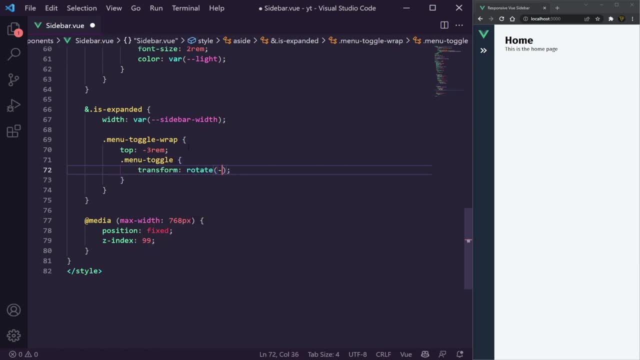 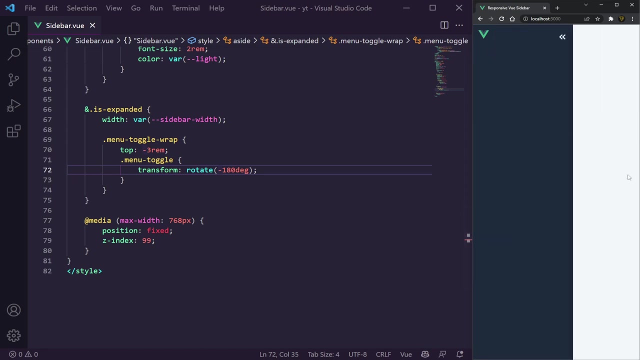 Element and we're going to say: rotate minus 180 degrees. Now the reason we use a mine is not just a positive is because I want it to rotate anti-clockwise instead of clockwise. So you can see that it now spins round and it's facing the right way, which is perfect. 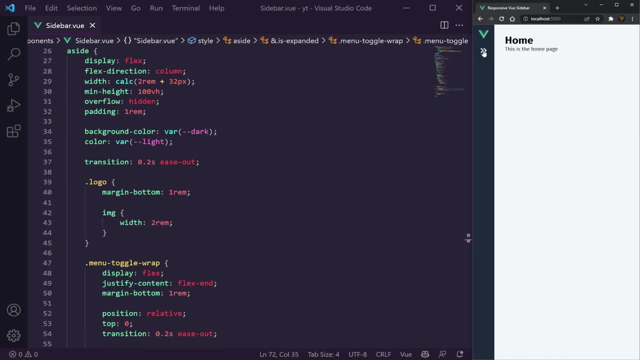 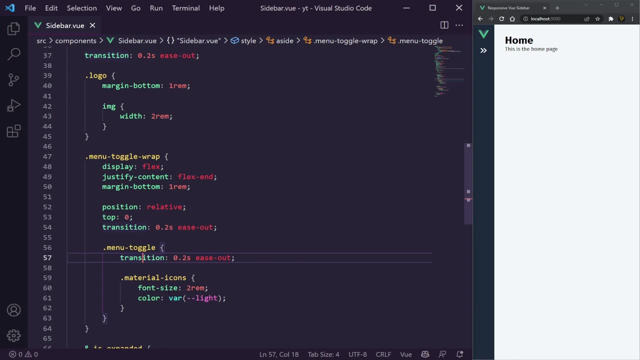 That's exactly what we want. I want to add a half per state to this. You can see, you can actually click it and it makes it a bit more clear. So inside of our menu toggle- here I'm just gonna go- The material icons. 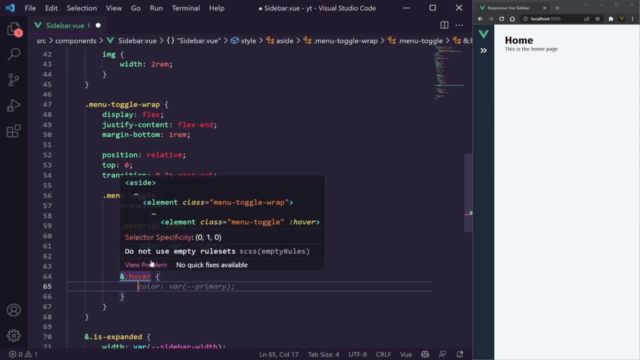 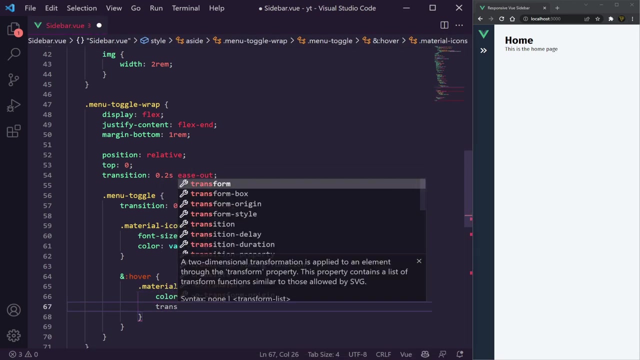 I'm going to say when we hover above this, if I have the day, you can see, it's say when we have on the menu toggle, we're going to give this the color or the sorry, the material icons, A color of far primary and water. going to say: a transform: translate X to be equal to 0.5 REM, which is about eight pixels. 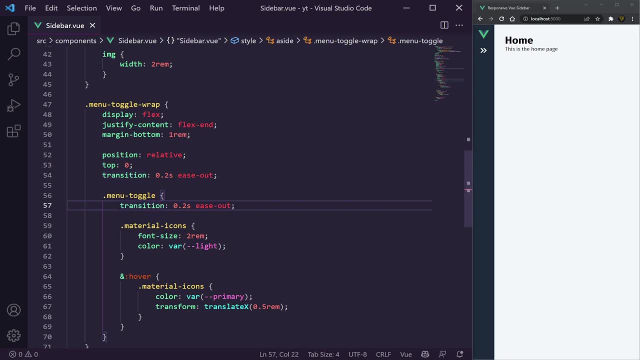 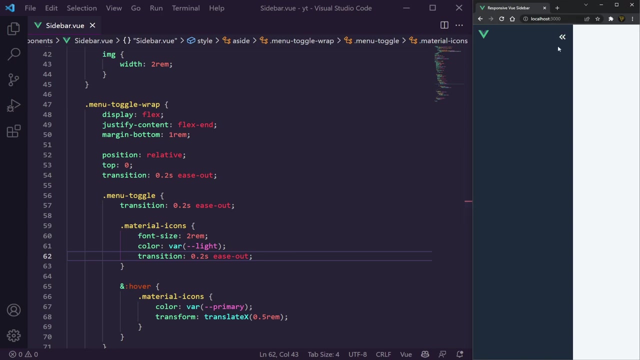 So you can see that that now jumps across. It seems that our transition is not working there. Oh, it's because we need to transition also on our material icon. And there you go. That's a nice little transition, And you can see when, once it's rotated as well, the animation works backwards and points inwards, which makes it look really nice. 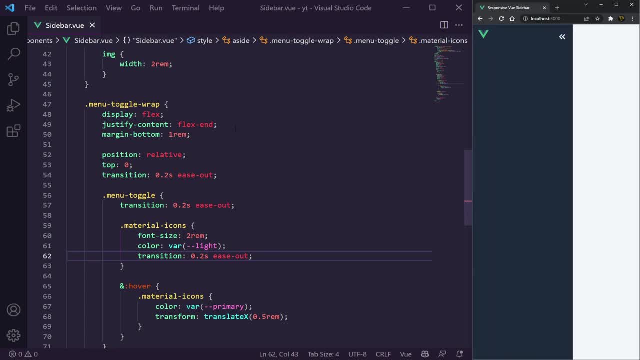 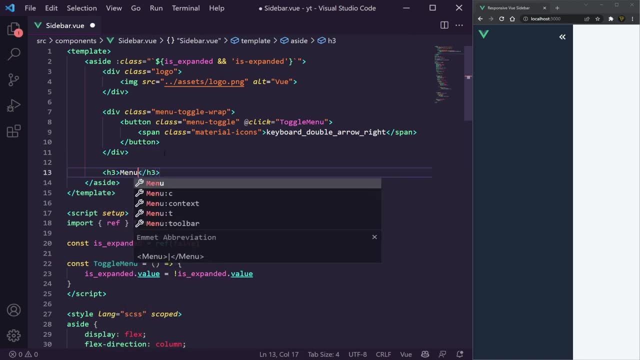 So that's that done. Now let's actually add in our menu underneath. So we want to go under here and we want to add in a hate free to start with, which is a menu, Just to identify that it is a menu, especially for those screen readers. 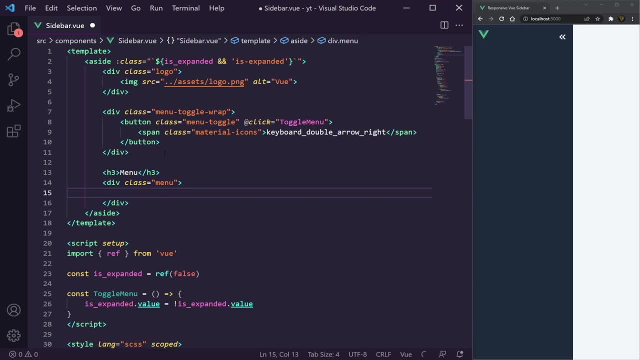 And then we can have a dot menu class, And then we want to have a router hyphen link with the class of button, and we want to do this about four times, So we're just gonna say four. And there you go. We have four router links with the class of buttons. 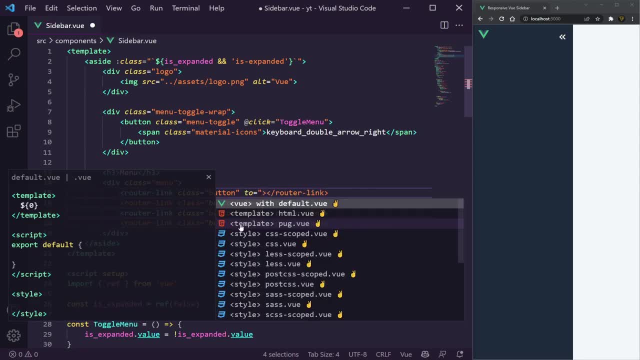 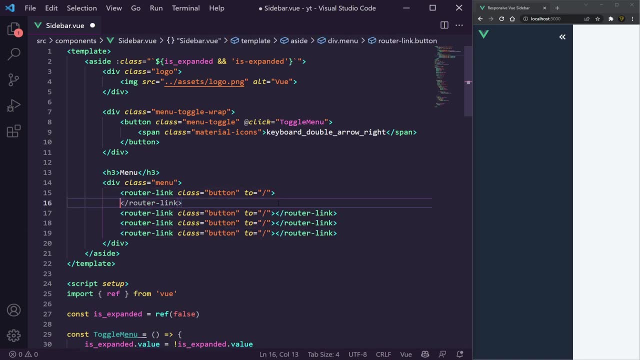 I'm going to add in a two to all of these. So there's a two. I'm just gonna say slash for now. And now in the first one, we're going to say home. Well, actually that's incorrect. Let's break that down. 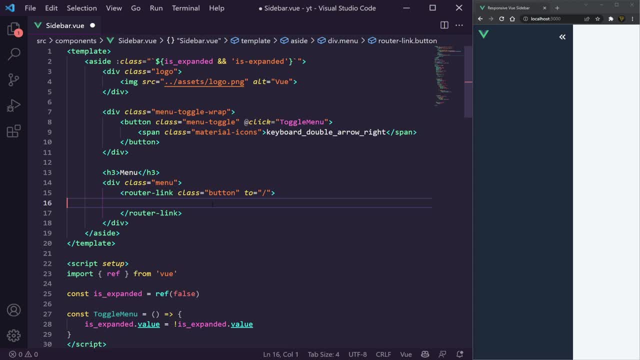 Watch you go. You know what I just realized? this is less close. all of that, We want a couple of things. We want a- well, there you go. We want a span with the material icons of home, which is going to give us a home icon. 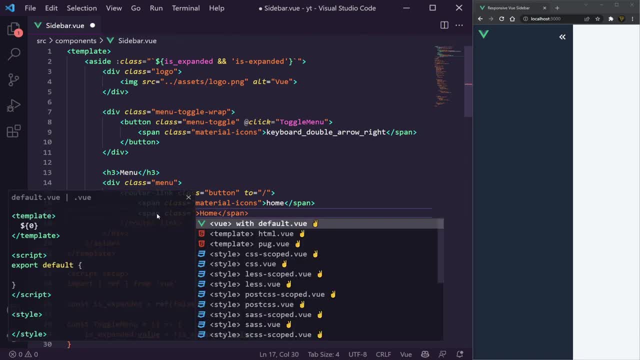 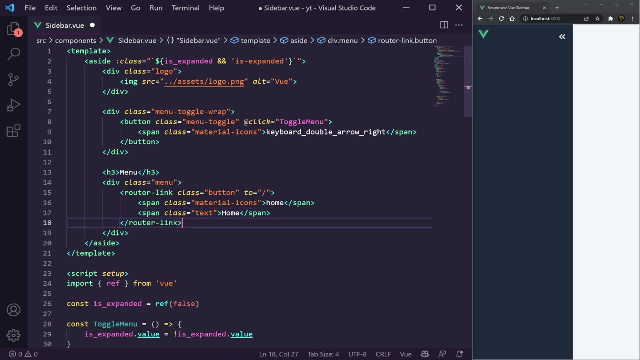 And then we want to give it a span with the class of text, equal with the class of text, So we can target this, this span, specifically there. Now we can copy this and paste it again And we can change this to, let's say, document, which is just one of the icons I'm using. 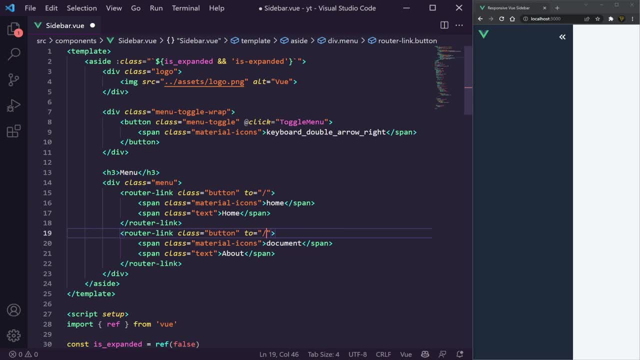 And this is going to say about, and this one is going to go to forward slash about, just like that. So let's leave that here And you can see we have two things here. It looks a bit ugly, but we'll deal with that in a second. 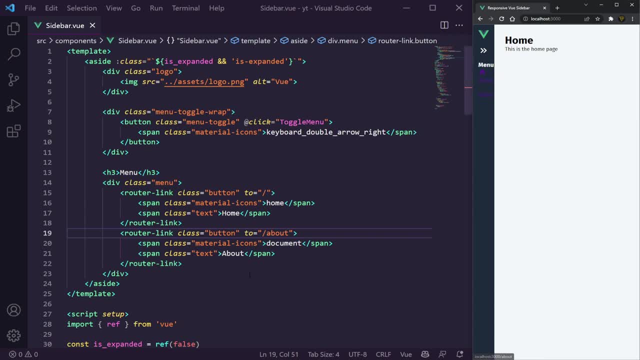 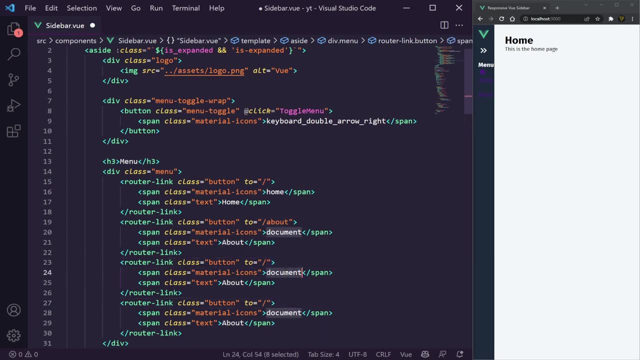 So if I hit about, you can see it changed to about and home takes us back. Now I'm going to duplicate this two more times, just so we have some elements. I'm just gonna leave these at home and this one will say: our team. 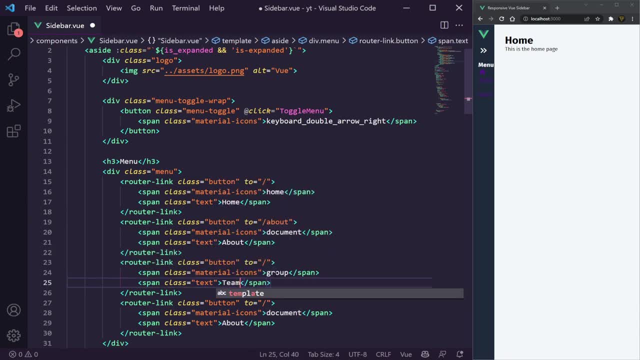 Oh, sorry, This won't be. And this one will say team, and this one, Why is it email? And this one will say contact us to save refresh, and you can see that the only one's not working is about: Let's have a look for an icon for about. 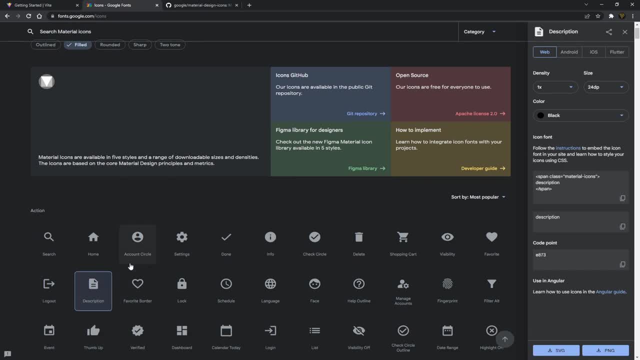 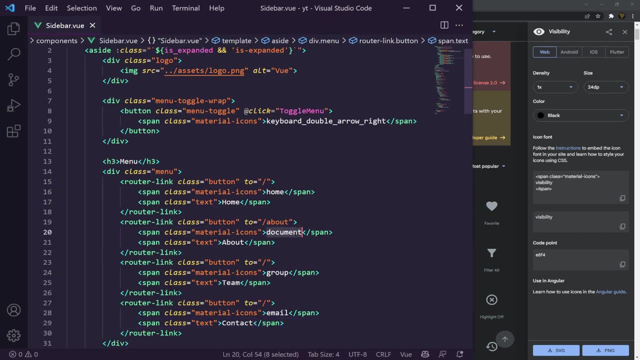 So here we can see a description. I think that's what we want to just do the eye. I like the eye. Let's do the eye. The eye looks cooler. I had a different in the actual the demo, but we're going to use the eye. 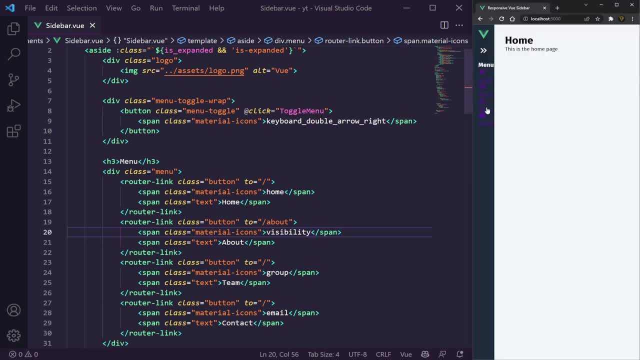 You can choose any icon you want. By the way, these are just the ones I'm choosing, And there you go. You got the about which the eye. Now it looks cool, but it looks really ugly, So we open this out. 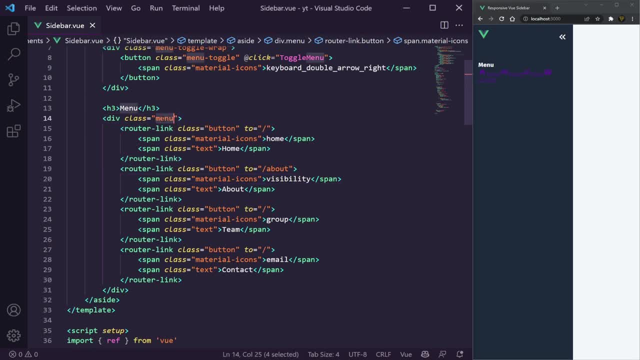 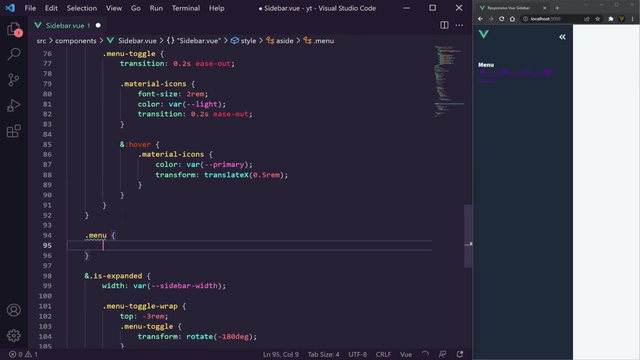 You can see it's all broken. It doesn't look very good. So let's go and style our menu to start with. So let's go in here underneath our menu, Toggle wrap will say: dot menu. Now the menu is going to be styled with a negative margin, which the reason we're doing this is because we want to add the padding to the actual element and not to 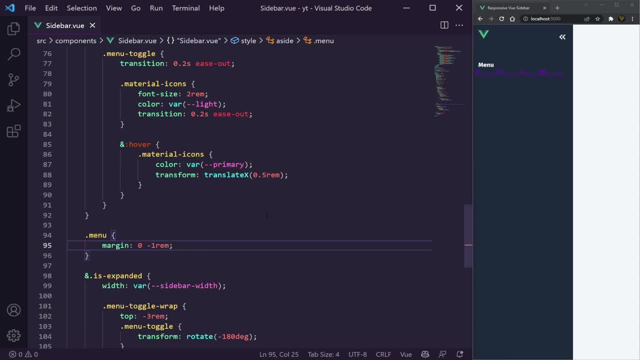 The not to not on the outside. I'll remove this and show you what it means later. We also need to start our hate free and our button Hyphen or button dot text as well. Now we're going to go in here, We're going to say opacity zero, because we don't want to be able to see the menu or the text when we're not expanded. 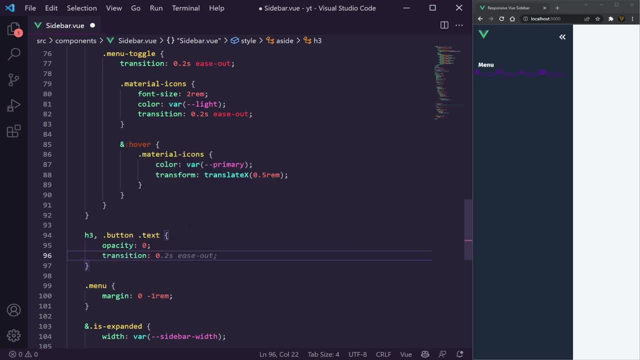 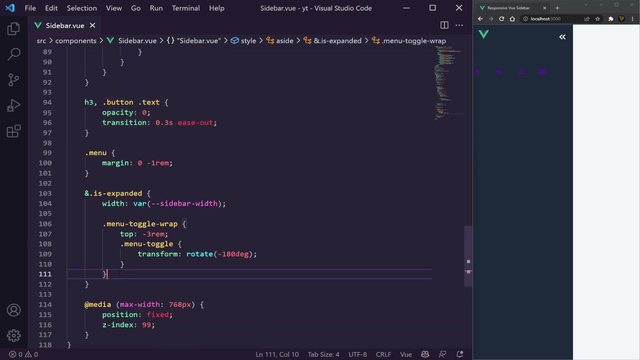 We're going to say transition, It's going to be equal to 0.3 seconds, a point second from the actual pulling out of the actual menu, And we just want to say ease out. like that We can then copy this, pull it inside off, our is expanded. 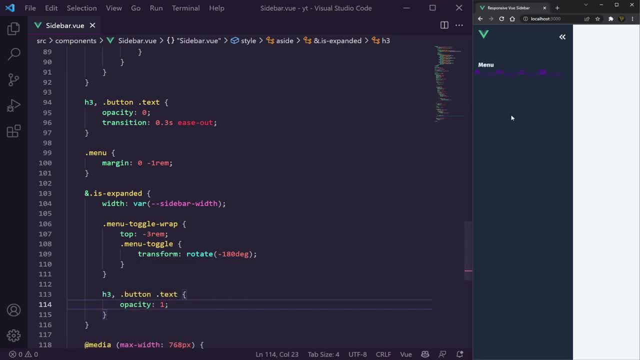 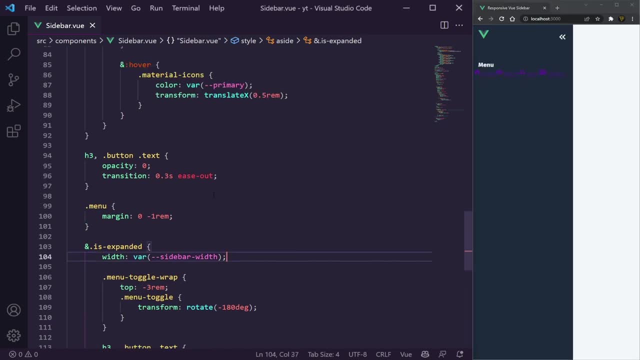 And I'm just going to remove the transition and said the opacity to one. And there you go. So now, when we close it, you can see the text is now gone and it's back, just like that, But it looks a bit broken still. 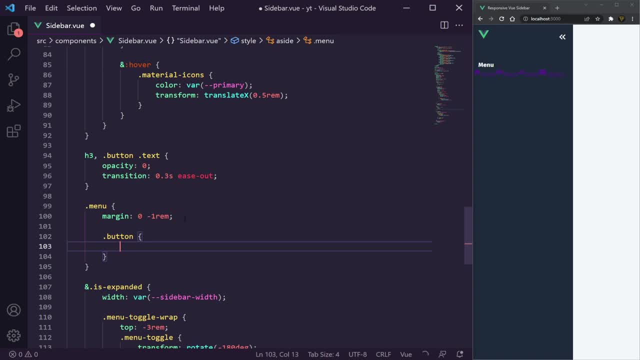 So let's go back to our menu. We're going to get our button inside of our menu and we're going to give this the display of flex. We're going to give this the line I am center and we're going to just say text decoration. 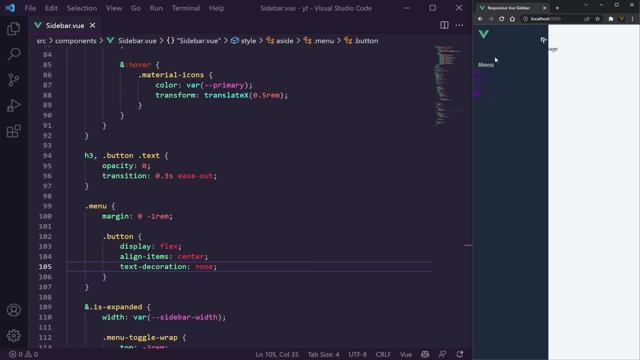 No. So we say, if you see us looking a bit better now it's, it's looking ethics in line instead of on right next week Offer. We're going to give this a padding of 0.5 round to one brand, which is going to basically be the padding to the left and right. 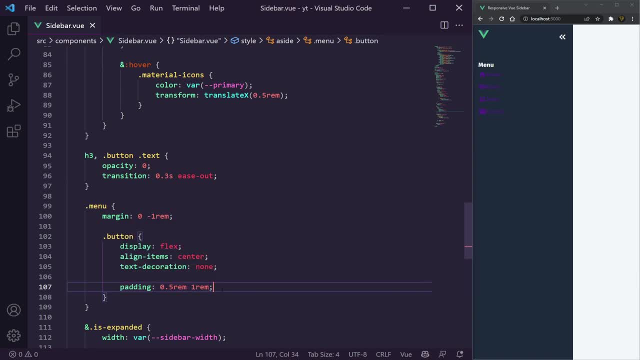 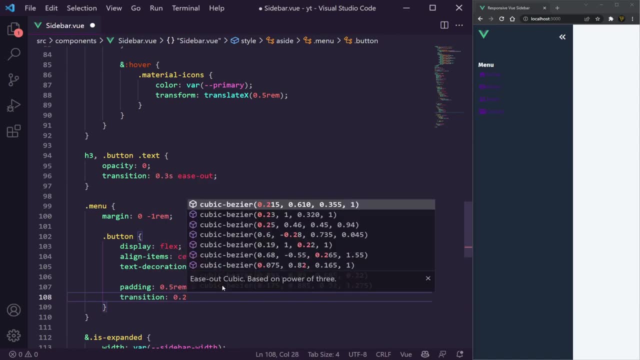 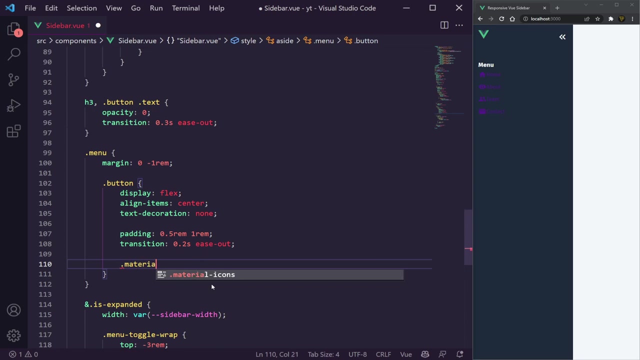 And then you're going to see, now lines up with this element here, And then, finally, we can Underneath the padding and give it a transition, transition off 0.2 or 0.2, ease out. We can then set the material icons to have a font size of two REM, which is going to be 32 pixels. 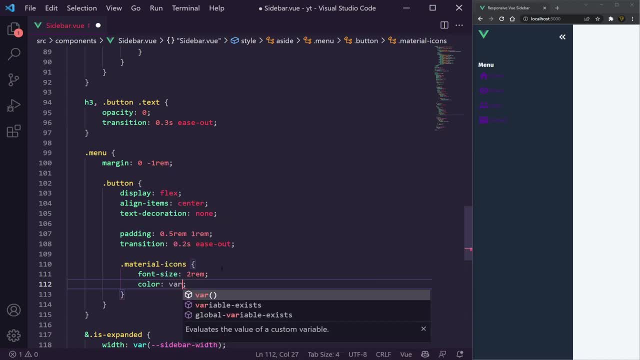 We can then also give it a color of light, far hyphen light And a nother transition on this. So when we hover over it we can have a state of 0.2 is out as well, And there you go. So that's the icon styled. 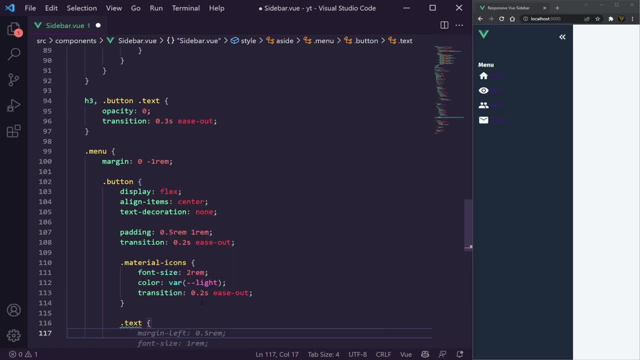 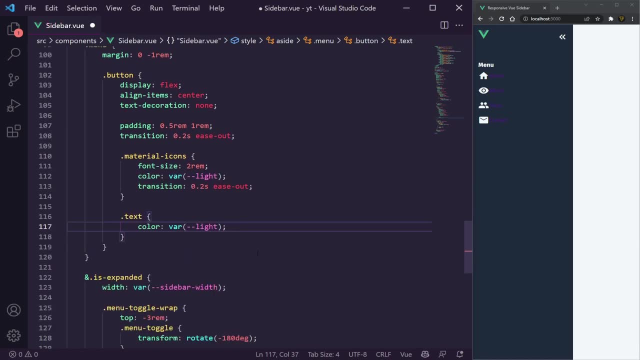 We don't want to get our text and we just want to really give this the color of far light. We don't want to give it a transition as well. We can copy this transition. I could have probably added this transition to everything, just to save time of rewriting it out, and it would make it more dry. 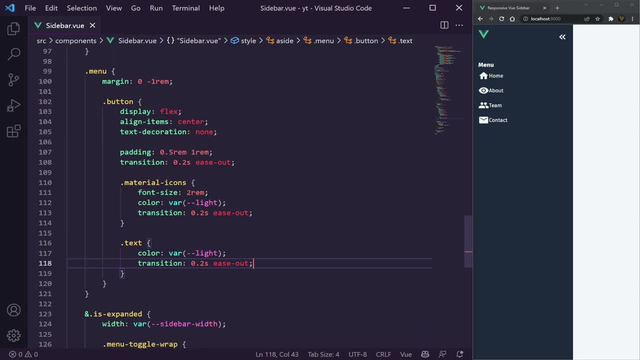 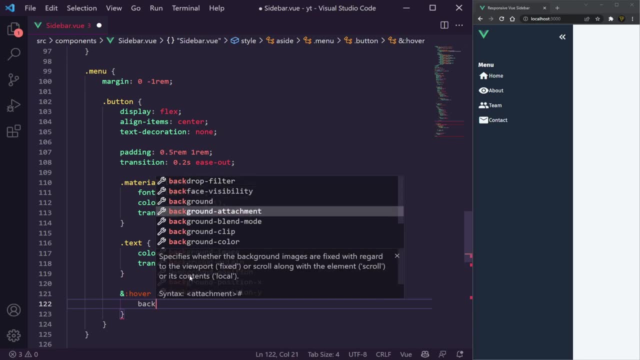 But also there's certain elements We only want to animate, not everything. So there we go, And then underneath this we can say: button on Hoffa. We're basically just going to say the background color is going to be equal to far dark old, which is the alternate dark color. 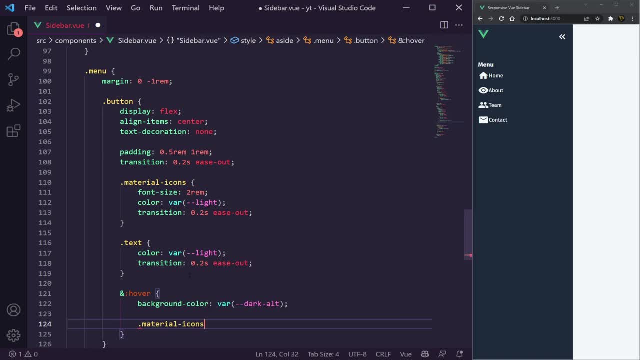 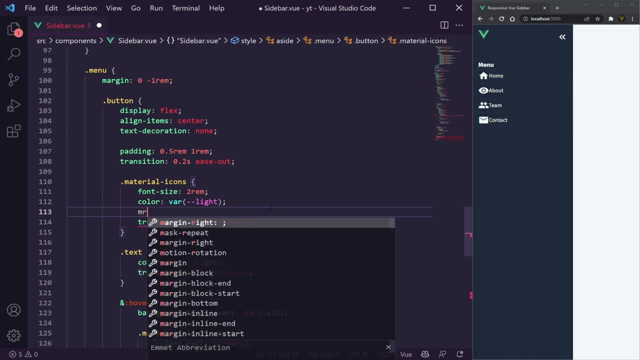 We set. but I'm going to get the material icons and the text. I'm going to set the color to be far primary, So when we're hovering over them, you can see here that now looks a lot better. Was it going to give this a margin right off one round like that, just to bring, give it some space away from it there? 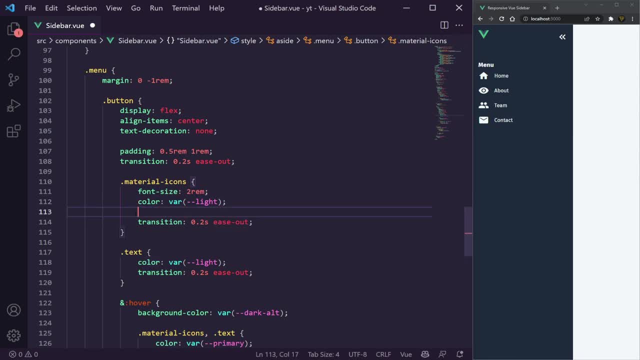 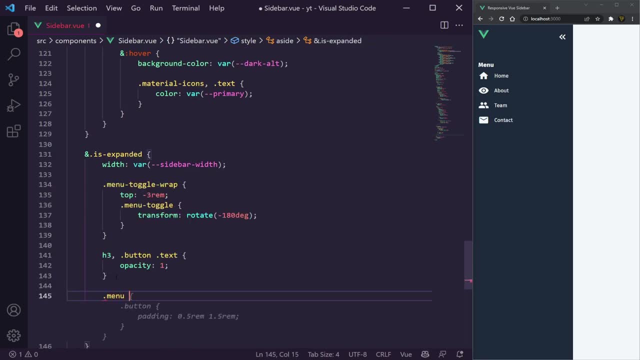 Well, actually, no, you know, we're going to take this away And we're going to go down to our is expanded underneath this hedge frame. We're going to set the menu And inside of our menu we just want to say, well, actually, no, we could just say button. 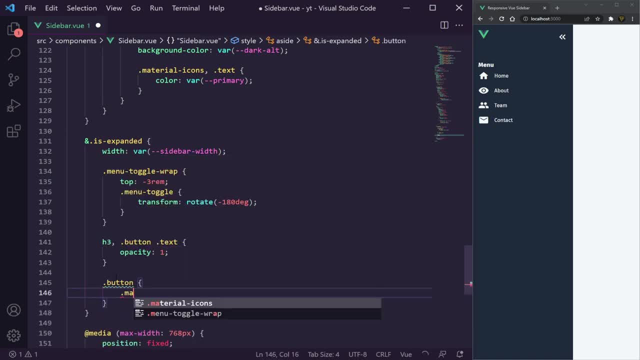 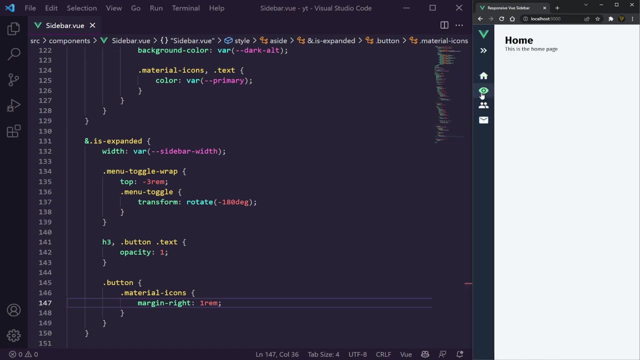 This doesn't have to be the menu, Say, our button and our material icons Need to have the margin right off one rent. So now when we show that close this and we open, you can see it has a sliding animation Like it's pulling itself in as well. 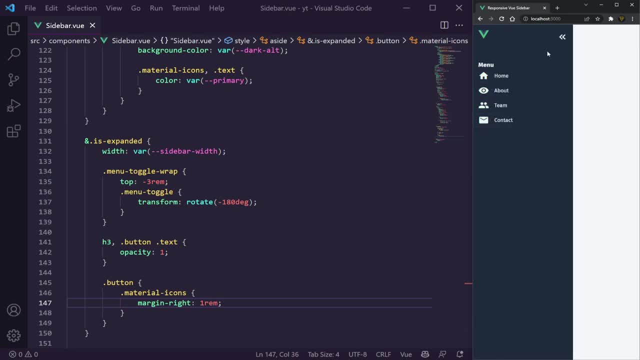 And there you go. That's, that's the base elements All set out there. It's looking pretty good. Let's add some more styling to this list, All this menu tag and a few other things as well. So we want to go up to a buffer menu. 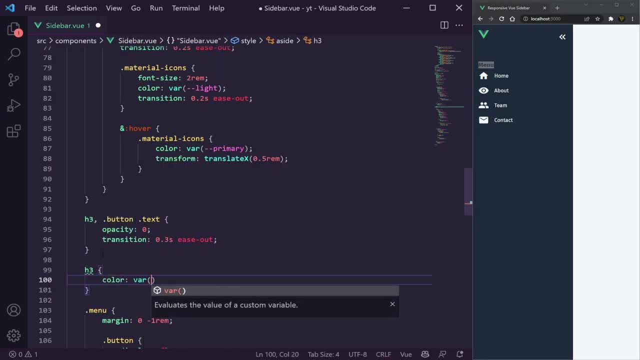 Just under this And there's a H free. We're looking for a color of far Ray. would they give it a font size? And we want this to be slightly smaller. It's a 0.7, 875 rent, which is about 14 pixels. 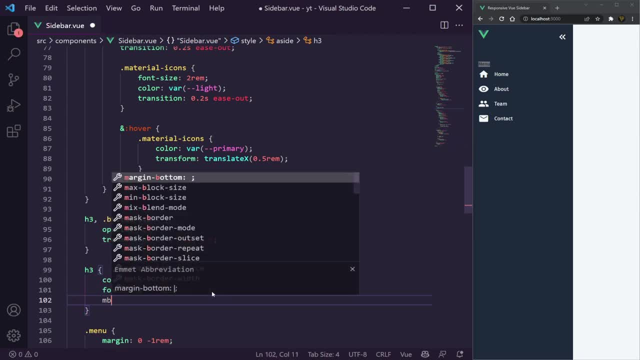 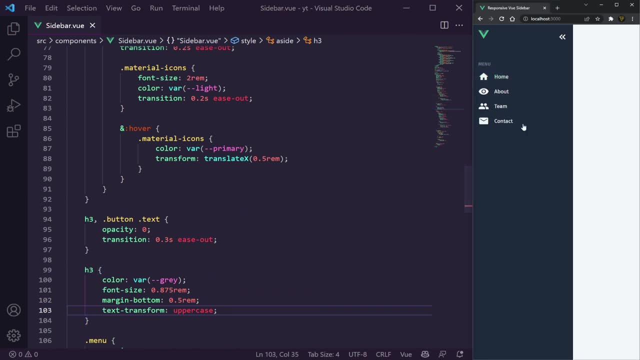 And I'm going to give this a margin bottom of 0.5 rent And a text transform of uppercase. So it's all capital And there you go. That's the menu Then. pretty cool, It's a nice little subtitle that you can see, but it's not too intrusive. 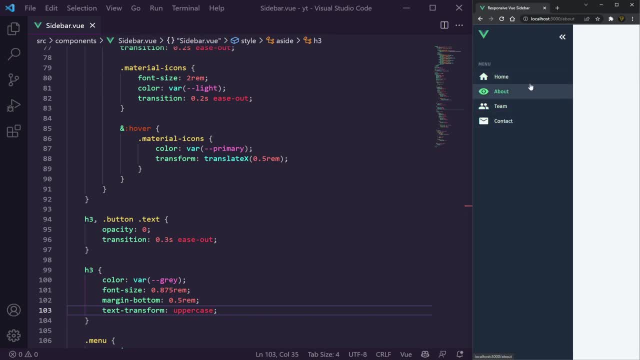 So it's out in another way. The next thing is, when we, when we click on the page, you can see it's not highlighting that page. It highlights when we hover, but not when we're on it. So we need to basically add in another class. 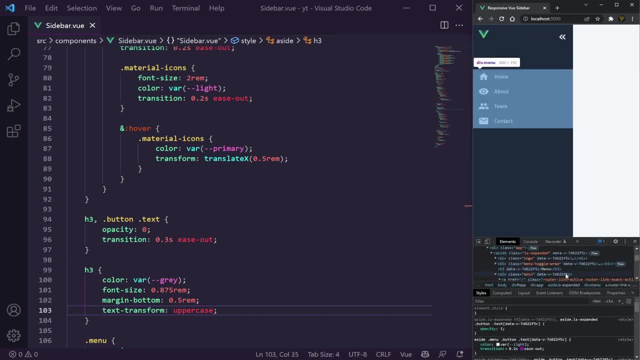 Now we inspect this here. You can see it's actually added some classes. You see the router link is active or we get router link Exact active. Now the difference between router link active and router link Exact active is router link Active will find anything. 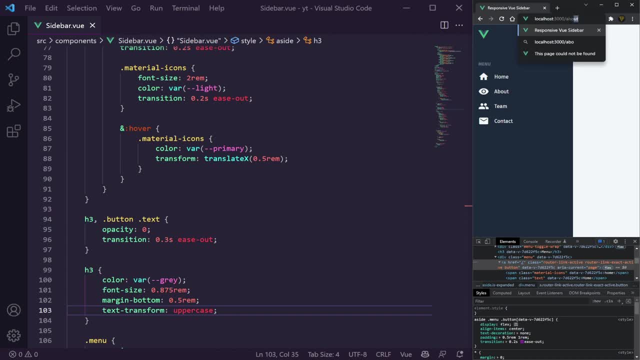 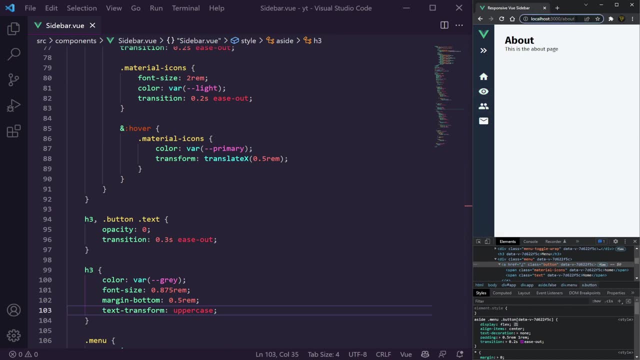 So let's say this was forward slash About, it would be on the about page but it also be referencing the home page. Or if we had about forward slash child off about, it would then be referencing the about page Still as well via the non exact method. 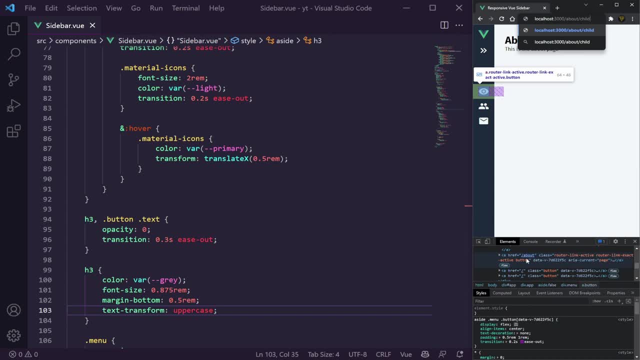 So the router link active, but router link Exact will only be on the exact link here in the hatred. So that's why we're doing that there, So you can see that. So let's go To our menu and in our button. 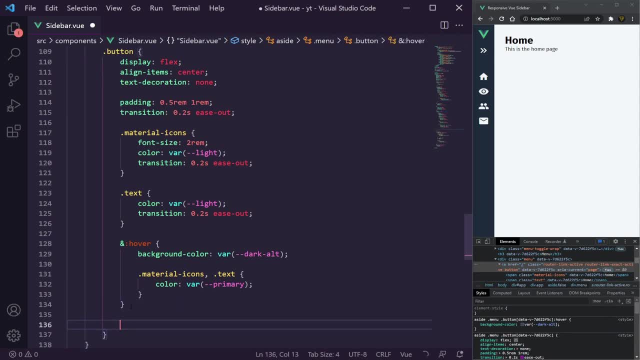 We just want to say, underneath all of this, under half off. Well, actually, we can actually go here and say: and this class now Safe, and that should hopefully when we're on the home page. Oh, we also need to add it after this. 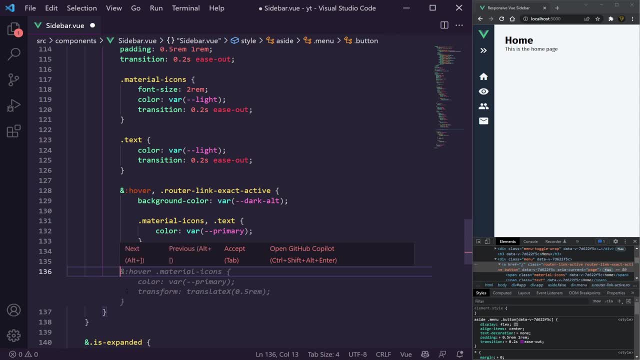 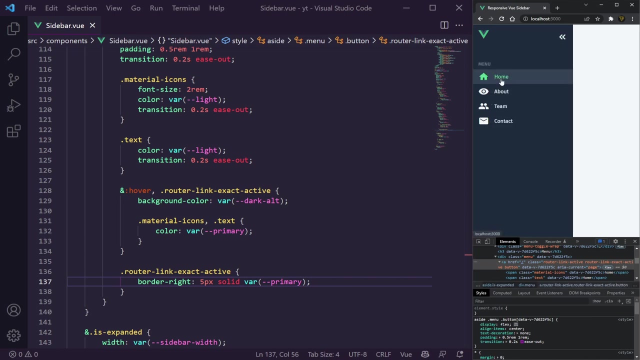 So we need to say: and material icons. So here we're going to say, when we just have the router active, we want to say: order right, five pixels solid and far. primary, It's safe, refresh and for some reason it's not working. 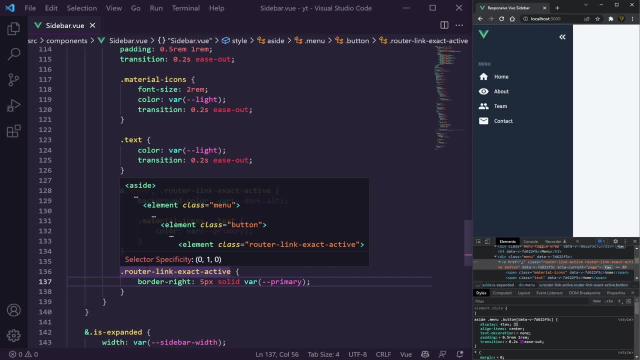 Now why router link Exact active? That should be right. Oh, you could see, here We need to use The hands and I also need to do, and there as well, It's safe refresh And it's kind of worked. 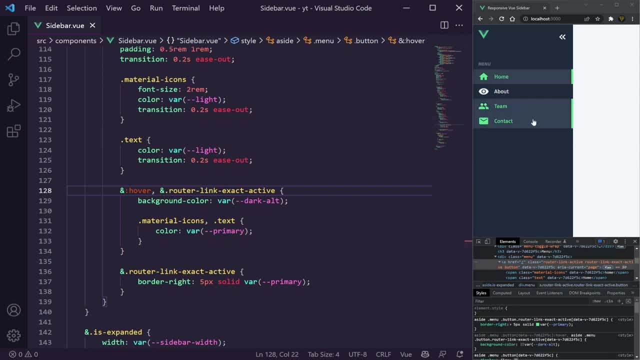 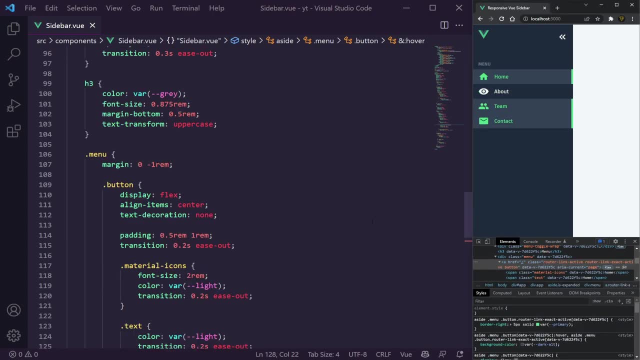 Oh, I did that safe. Okay, so that's kind of working. except you could see everything is highlighted except the about page. We select the about page. It works. Oh and guys, I've just realized why it's hotline. 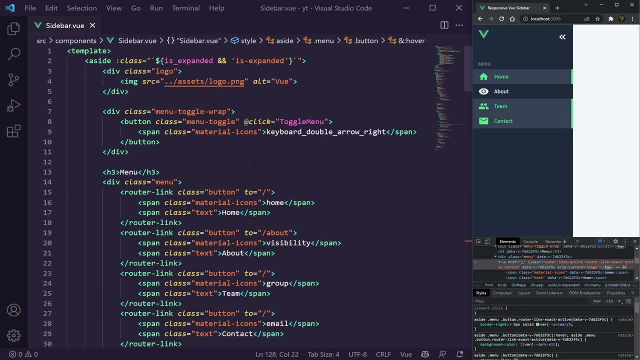 Every single one is because inside of our sidebar we have them all set to this forward slash, So we just need to change these ones to say so it goes. Let's just say We can have team and then the one below is going to be contact. 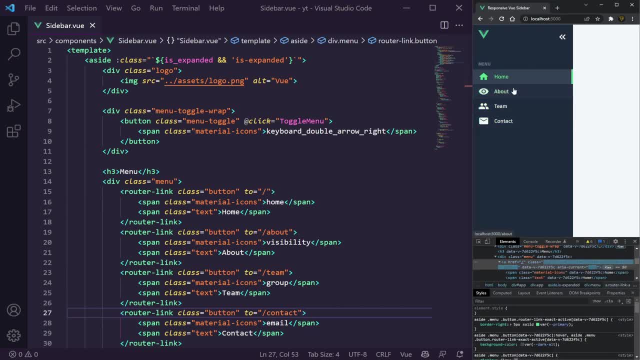 It's safe. And there you go. They're no longer highlighted. I can't believe that. took me a minute to figure out. But there you go, She can see, we can have her. and these have little animation to actually bring them. If you click on these because they don't actually exist in our router, they actually just throw errors in the console here saying there's no match for it. 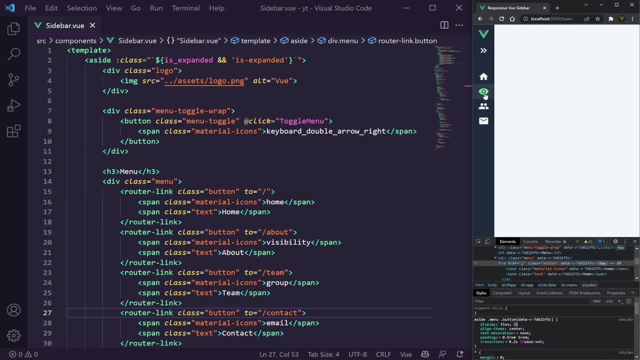 So just so you know, that's what happened. if we shut this as well And now we go home, It's his home page, We swap, It, says about, but you can obviously see that That's on mobile. If we now make this bigger. 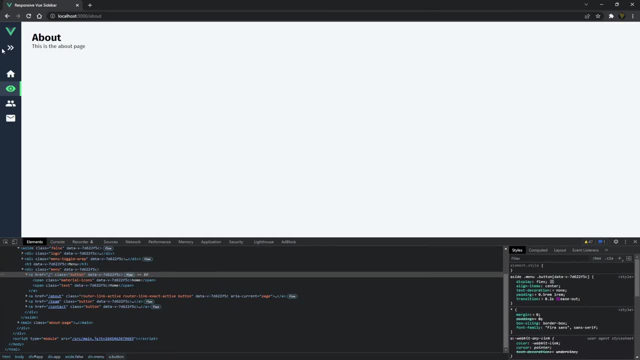 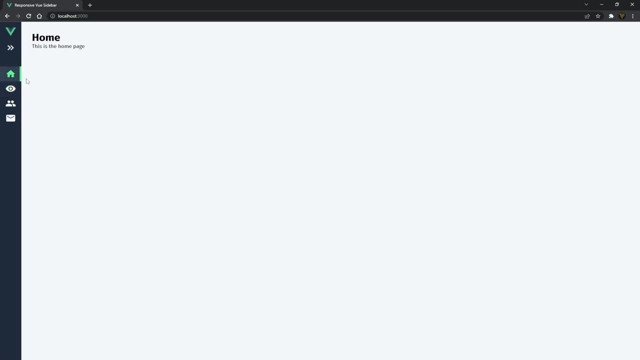 So if we bring this out and let's just slam it to the top and we open this, you can see, instead of obviously this being behind it, It's now to the side of it and we can show it and it will follow it exactly, which is really nice. 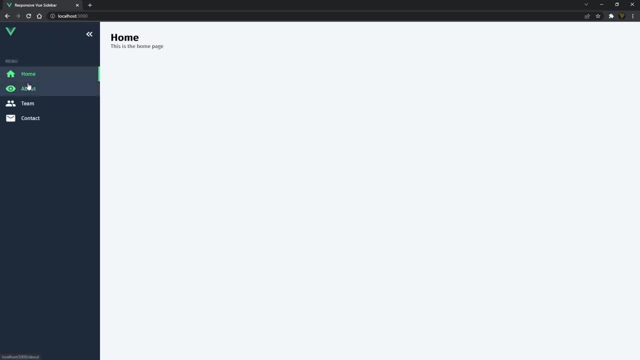 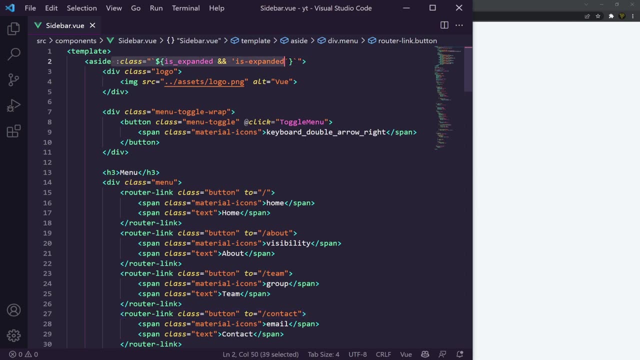 And it looks really cool when we have it both ways. So nothing is. we have a settings burn at the bottom here. Now how do we get burned from up here to the bottom? Well, we actually added the class to this called Flex. 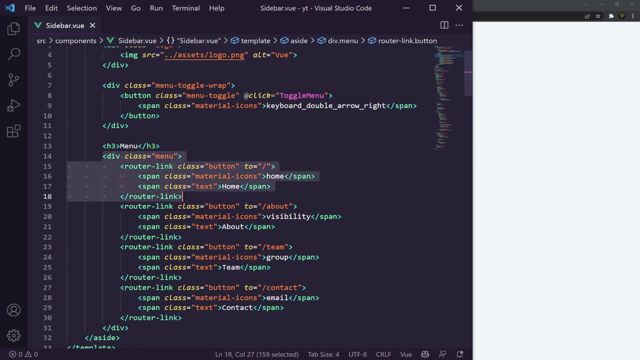 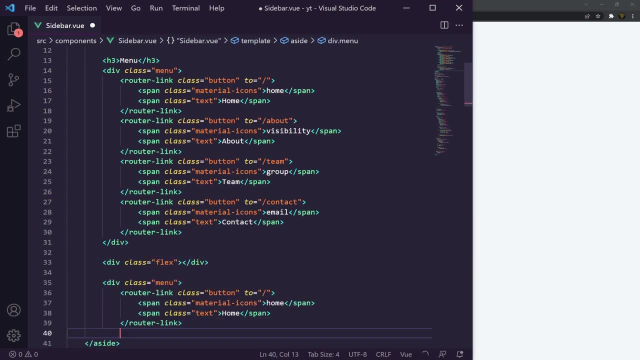 which allows us to push Things around. So if we was to copy this menu and this round to tag, go under here I'm going to add a class called Flex, But then under this, I'm going to have in the menu which we're going to set to settings, settings, settings. 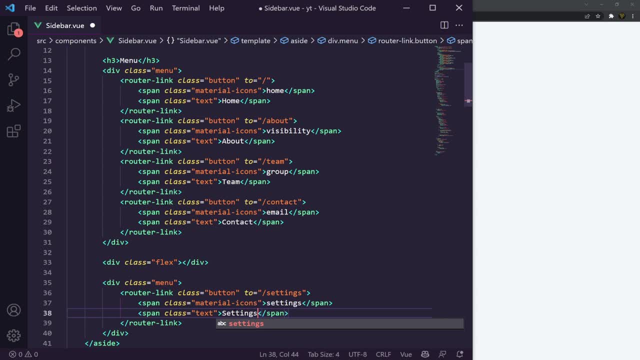 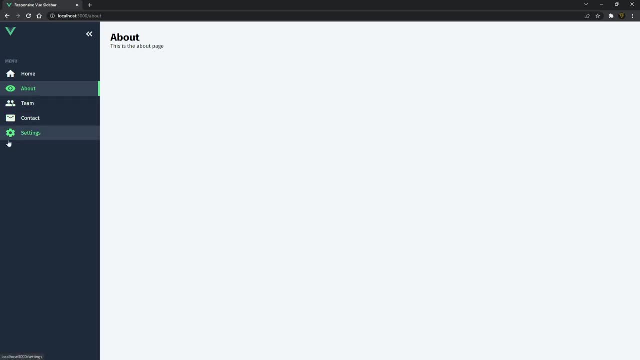 And this is going to say settings, just like that. And now we refresh. You can see this sex is there, but it's underneath of. how do we move it down? So we're going to do that by going Into our CSS, scrolling right down to, let's say, below: 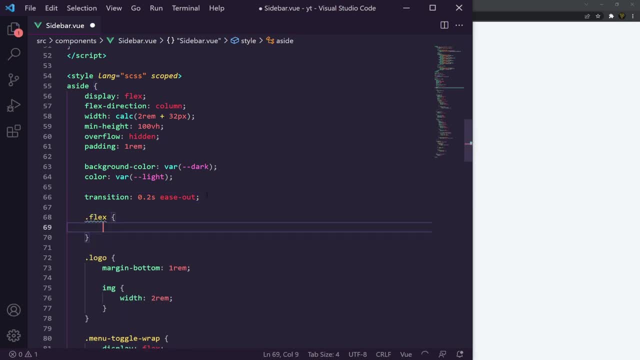 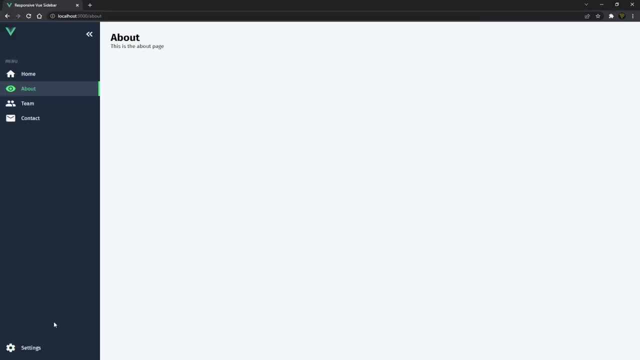 Well, you know, we could do at the top here, just under here, We can say: adopt Flex element is going to have flex one, one zero to push it all the way. And there you go. You can see that's pushed it down to the bottom. 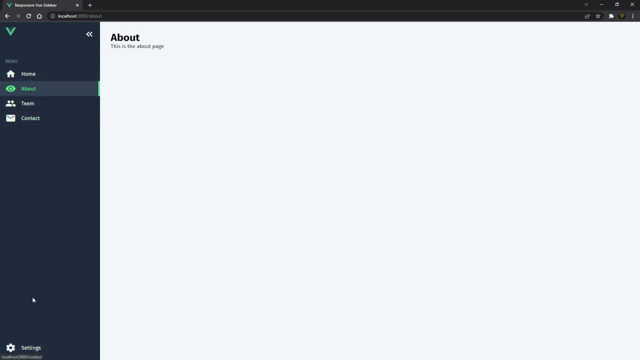 Now it's down here. So that's how we can move elements straight to the bottom and give some spacing in between And there you go, So that's flex out, You can sort to home and now the menu you can see works really nice. 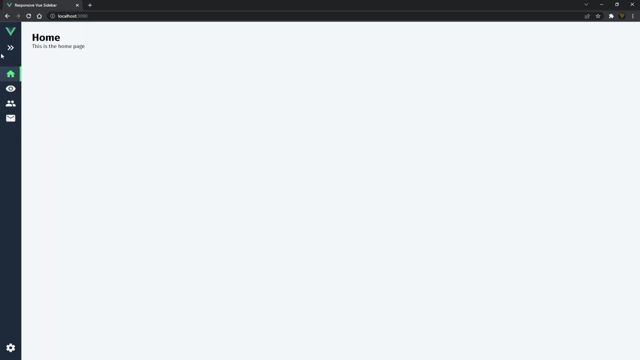 Everything pulls out. and that's there. Now there's one last thing. If I refresh this page, you can see it goes back. If I refresh again, it goes back. Now, how do we add local storage to this to remember the choice we make? 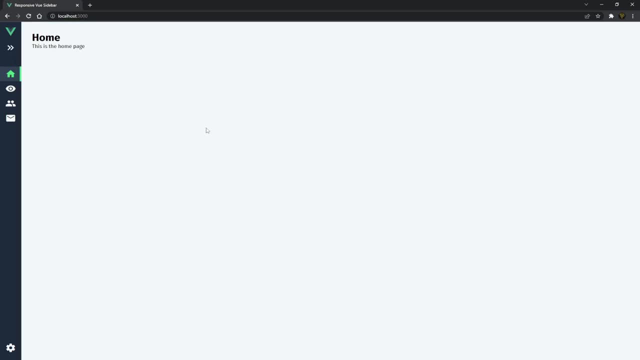 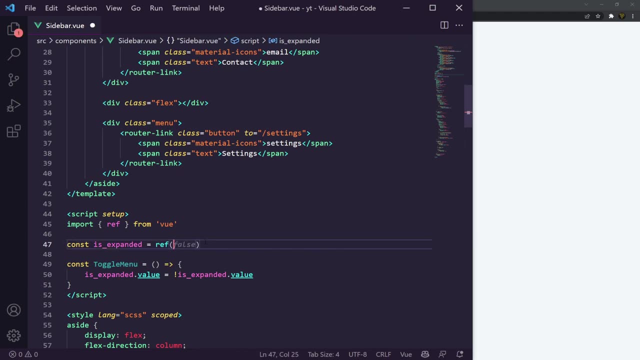 So if we want to open and we refresh, we want it to stay open, just for the user experience. So that's super simple. inside of here, We're going to change this ref false to be ref local storage dot get item And we're going to get this underscore expanded. 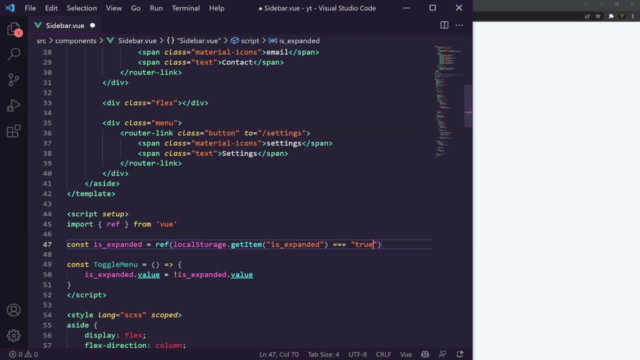 And I'm going to check if it's equal To true. If it's equal to true, then this is going to return true. Otherwise, if it gets anything else like null or undefined, it's going to say: or even false is going to say it's false. 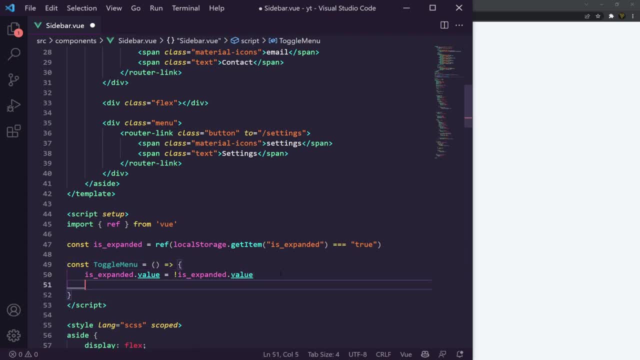 Now to set this when we toggle the menu, all we have to do is underneath this week, Say, local storage, dot selling is expanded by expanded dot value, And that's going to save the state of our things. And we refresh, and we click this, and we refresh. 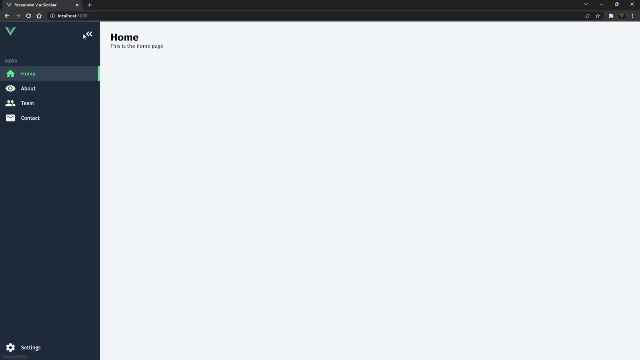 You can see it's now saved. It's open. If I keep refreshing, it's always saved. If I show it and refresh again, you can see it's now saved in the shut state. that will always remember what you're doing. Unless you clear your local storage, it will always remember what that is. 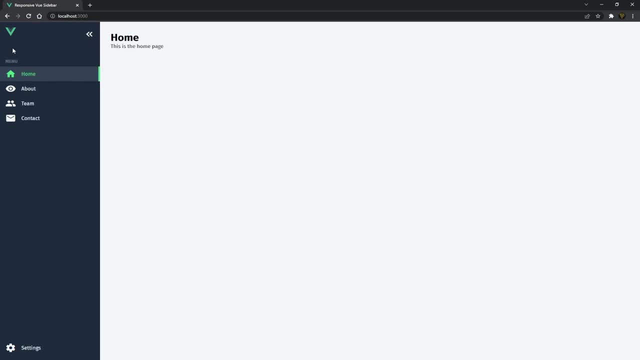 And that is it for this tutorial, guys. It's super dead simple, super straightforward And, as you can see, it's pretty awesome to create this super simple, mobile, mobile, responsive as well. So we move this to the right side and we just do this. 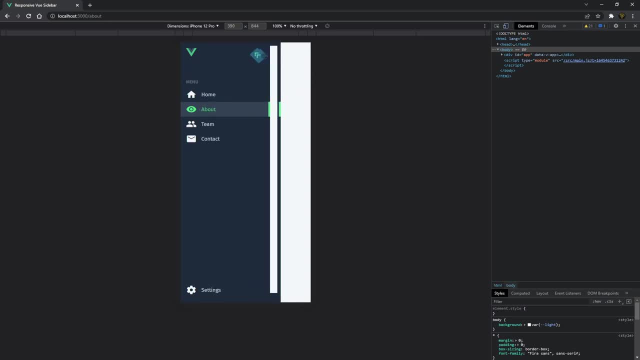 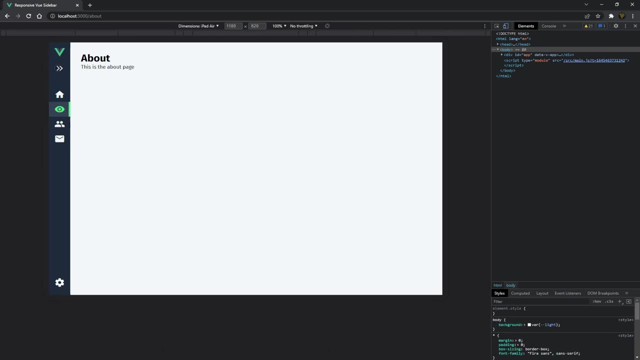 You can see it works on mobile And it doesn't push the content to the side and break it. It goes above it. Let's say we go to the iPad Air, You can see the menu still works, And if we go to the long mode it's looking good as well. 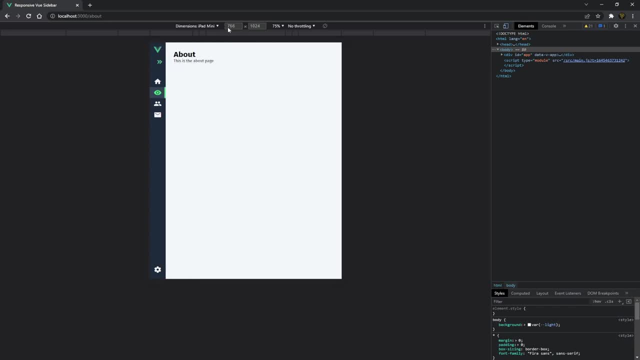 If we go to the iPad Mini, you can see it goes over above it because it hits that threshold of 768.. Because I'm pretty sure the content would be way too small in this side if you didn't. But you can see there how it's all working, how it would work. 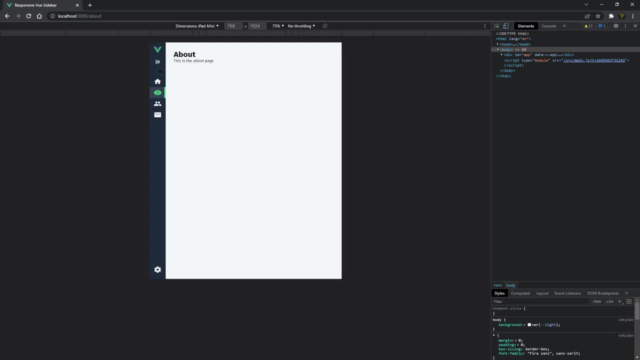 Now there'll be. there'll be some, probably some- extra challenges you need to accomplish, To think about when you actually create more content in here, But otherwise this would work flawlessly And you just have to make a few tweaks when you actually add content to these pages. 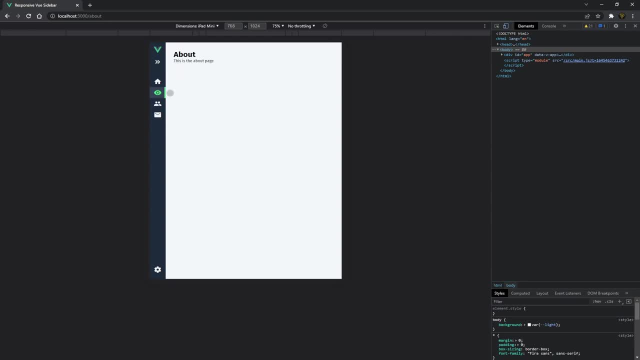 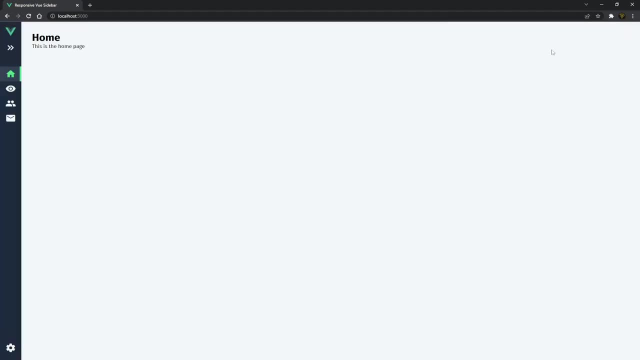 Otherwise it depends on what content you actually add, So you can't really cater for every scenario. But, as you can see, that is what we've been built today. I hope you have learned a bunch of cool things with Vuejs. If you have, don't forget to leave a thumbs up. 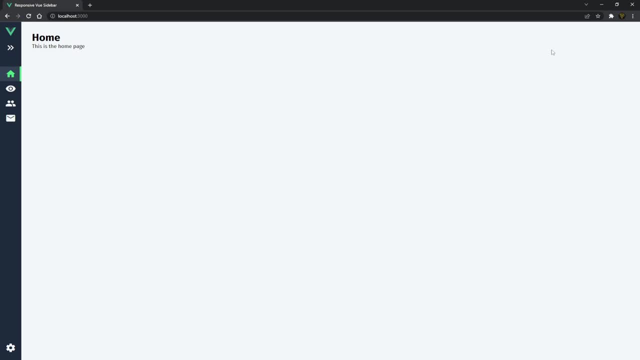 It really helps out my channel and I really do appreciate it. If you're new around here and you do want to see more, consider smashing that subscribe button, Joining my awesome community of developers and learning with us. I'm still learning myself, to be fair. 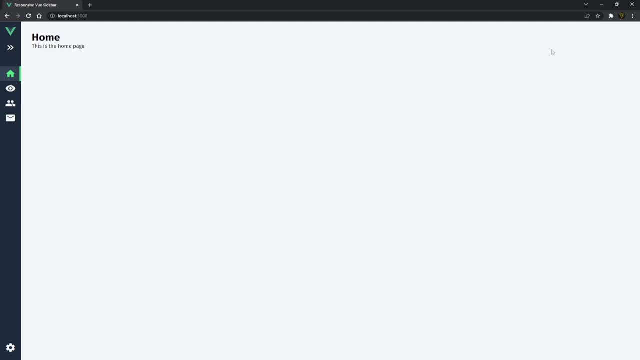 I just make it up. as I go along, I come up with an idea. I'm like I'm going to record that video and we do it, And that's how we create these cool videos. So don't forget to subscribe if you want to see more of that.